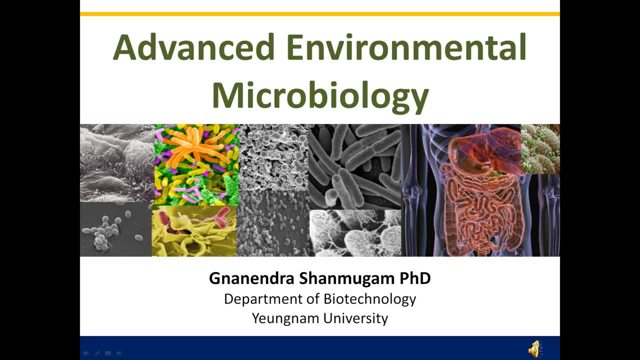 data analysis methods to handle. this large-scale data provides an exciting opportunity to explore, to understand the microbial communities from various environments like water, soil, plants, animal tissues and even space and many artificial space labs. spaces react by like bioreactors, so this kind of analysis really helps us to know who are present and what are they doing in that. 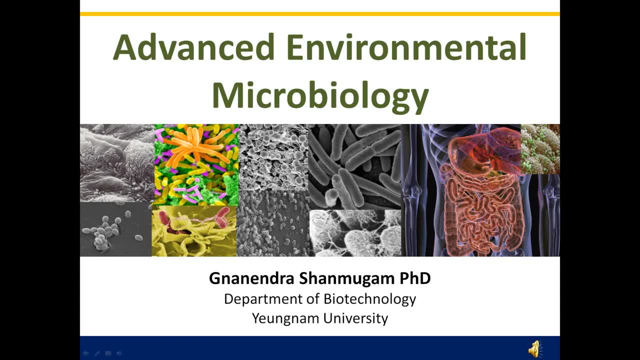 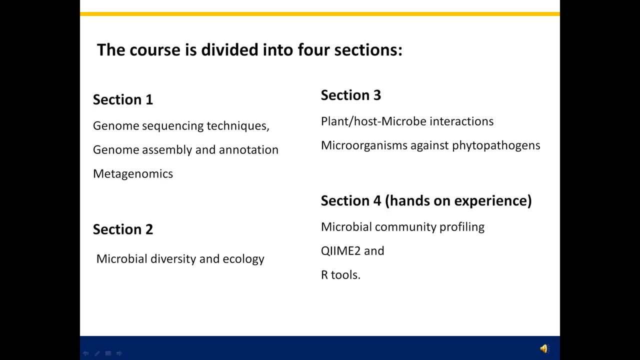 community. so let's have an overall look about what is environmental microbiology and what kinds of data are available for us and how we can handle and analyze those datas in this course. so coming to the course content, the course is divided into four sessions. section one deals with genome sequencing techniques. 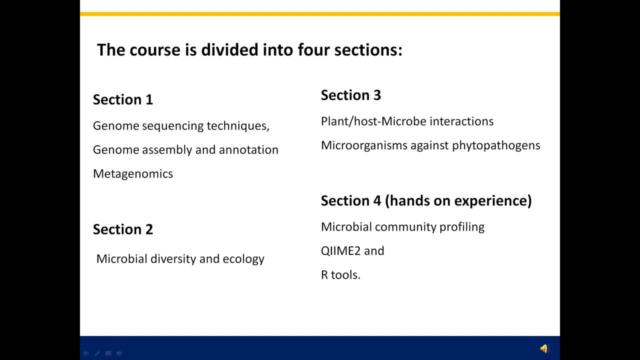 where we are going to deal with various sequencing technologies, library preparation kits, data analysis platforms and genome assembly and annotation. so where we are going to see- and various annotation pipelines and genome assembly tools and and metagenomics. so what are the preparation methods, what kind of data we can get. 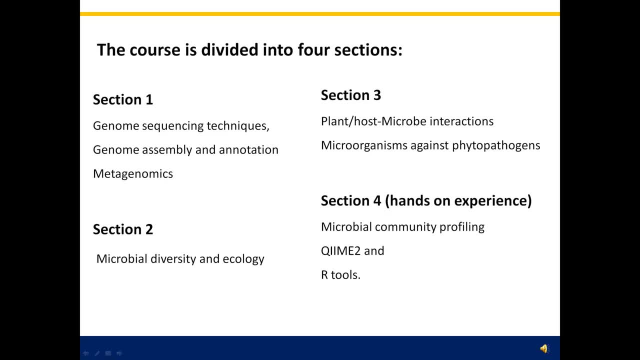 and how we are going to analyze that when coming for in section two. this deals with microbial diversity and ecology, so which is mostly about an microbiome data. and coming to the session three, it deals with plant and host micro interactions, so how the microorganism has been beneficial for the 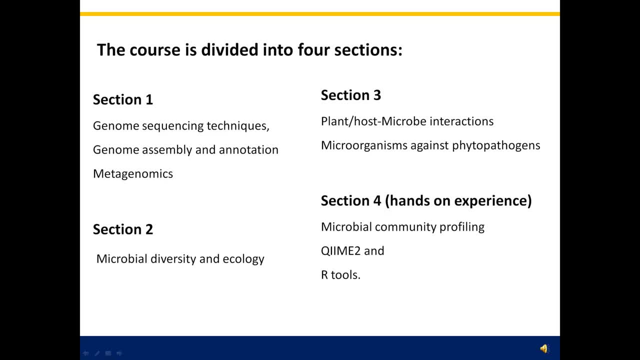 plant or its host. so we are going to discuss a few things about that. and microorganisms against phytopathogens: so how the beneficial microorganisms are helping the host to fight against the invading pathogens. and coming for and session four, so this will be an hands-on experience, so where we are going to deal with and certain microbiome data, so which? 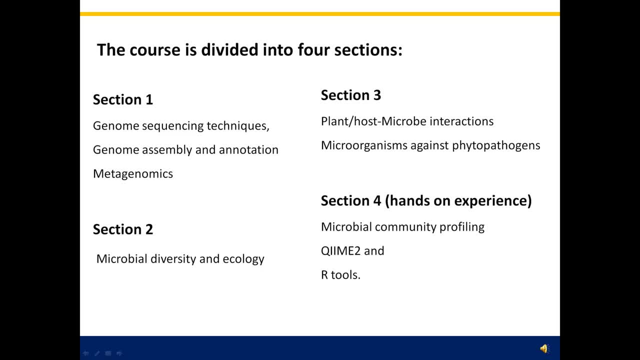 will be available from an source, from an mcbi or from open sources. so we are going to deal with and specific microbiome data and we are going to make an community profiling for that by using and chime tool, chime tool and we are going to use an r studio for making a beautiful graphs with an. 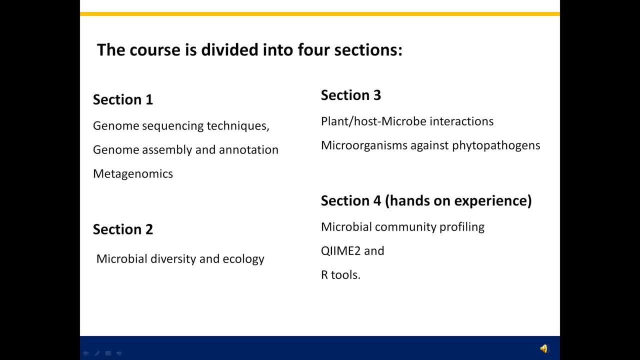 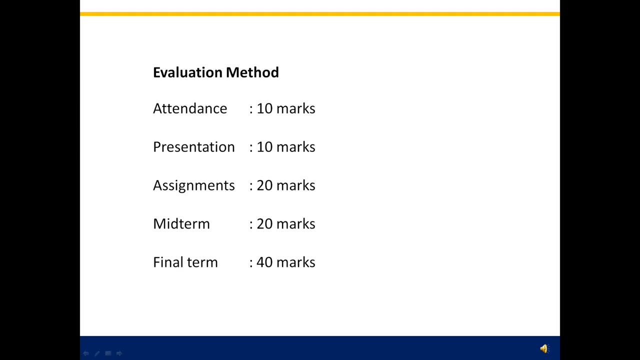 plotting or publication ready figures by using an art tool. so this is all about. and course content, so which we are going to discuss. so this will be. and for session course. so the course evaluation method is based on five different categories, like attendance, presentation, assignment, midterm exam and final time exam. so each has been distributed. attendance: 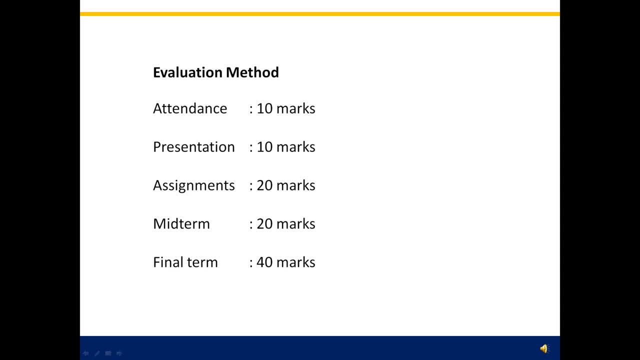 presentation is carrying in 1010 marks each and assignments 20. so overall it says the two assignments each tension marks and midterm is for 20 marks and final term is for 40 marks. so overall this is an evaluation pattern which is based on five different categories. so this is an evaluation pattern which i am going to follow to 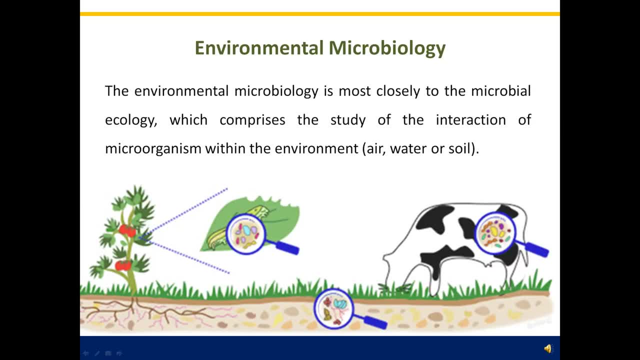 evaluate or to graduate to grade u students. environmental microbiology is most closely related to an microbial ecology, which comprises the study of the interaction of microorganisms within the environment, like air, water or soil, so this environmental microbiology is also defined as study of microbial interactions and microbial communities in the environment. 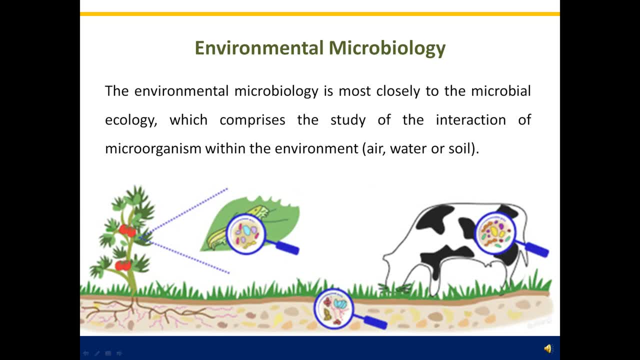 so usually this environmental microbiology deals with microbial communities that are helpful, how they are making and element cycles and biogeochemical processes and what are the acronyms that have been seen in extreme conditions and what are the microorganisms that have been seen in. 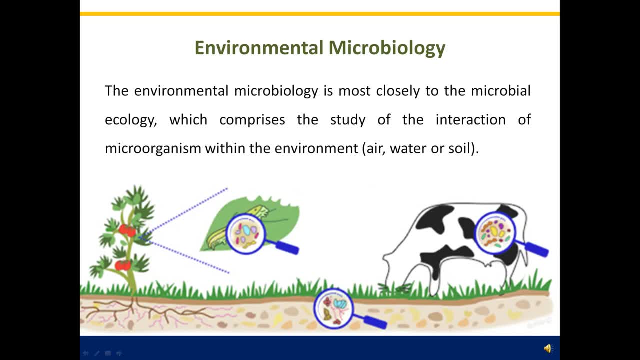 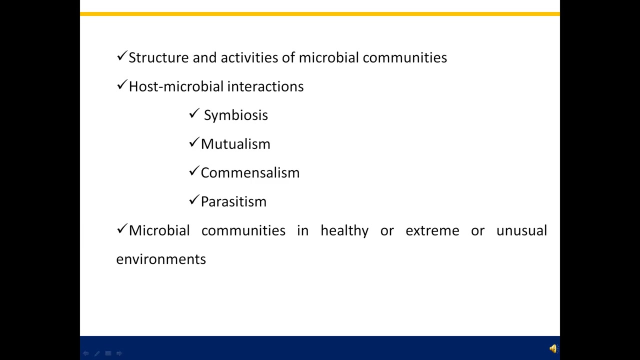 Different habitats, like terrestrial microbes, aquatic microbes, extremophiles, and that lives on different organisms. So these are the various studies which deals with an environmental microbiology. So structure and activities of microbial communities host microbial interactions in which we are going to see about symbiosis, mutualism, commensalism and parasitism, and microbial communities in healthy or extreme or unusual environments. 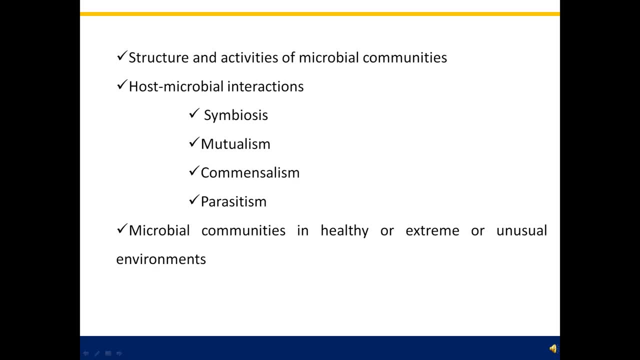 So coming for an structure and activities of microbial communities, this usually deals with which phylum is rich in community and which is not. So what is dominant at specific conditions and what is the role of those specific bacteria. So we are going to say that, okay, what is the structure of this particular community in this particular conditions? 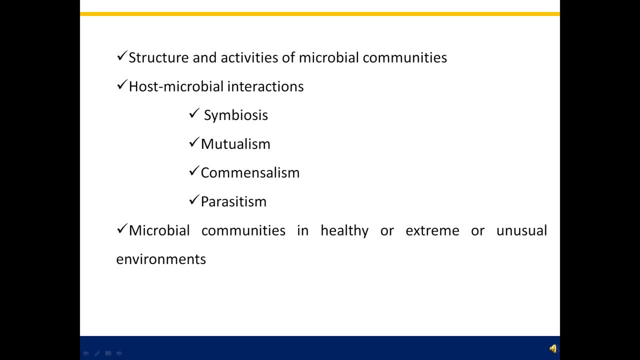 So what is the community which has been present in another comparative condition Say, for an example, like I want to find out the structural communities between healthy plant and then draft condition grown plant, So we can compare that okay, in healthy plant, So in a natural soil plant, so which phylum is rich and which has been dominant, as well as in draft region. 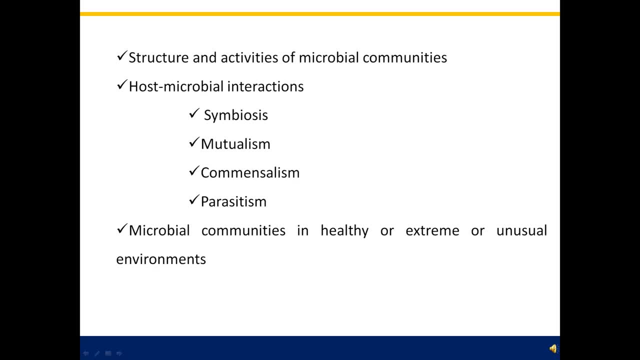 So which microbial phylum is rich and which is dominant? So, and what is the role of each and every bacteria? So we can compare that. So that's in structure and activities of microbial community And it's coming for an host microbial interactions. 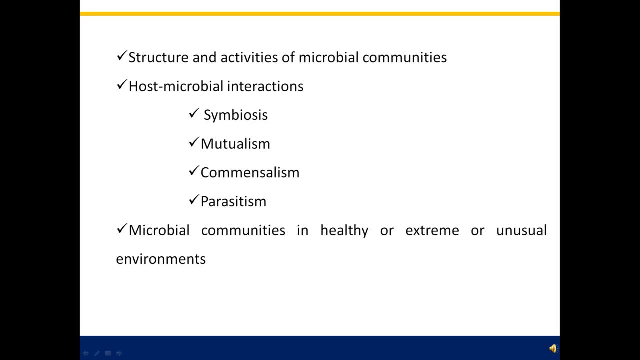 So here it deals with the nature of microorganisms and its interaction with its host, Say like whether the microorganism exists as symbiont, mutualistic or commensalism or parasitic in nature. So say for symbiosis, so this is a relationship in which one organism may depend on another for its survival. 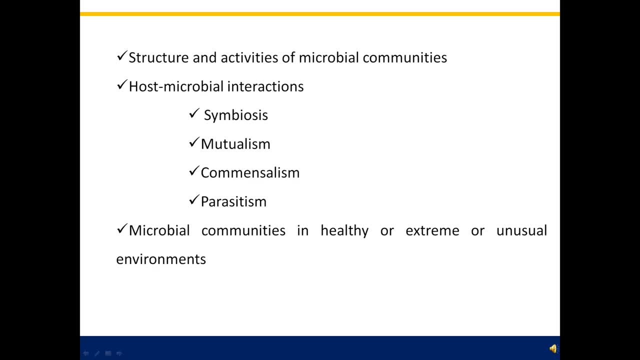 Sometimes they need each other, So mainly they rely for food and nutrients. So that's in symbiosis and mutualism. So in this type of relationship Both host and microorganisms gets benefited, Say for example E coli, which is synthesizes vitamin K in the intestine of host. 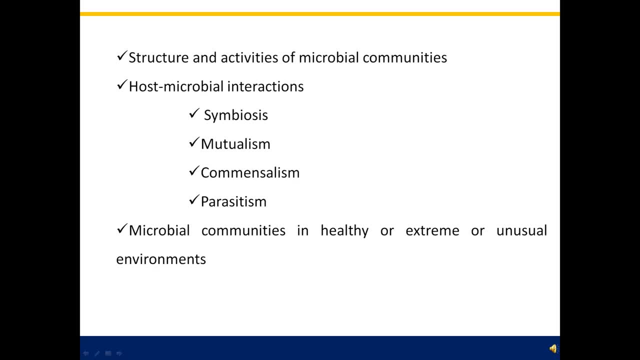 And mutually it's get benefited by getting a nutrients from the host intestine for its own survival. So next coming to an commensalism. So in this relationship one organism is benefited and the other is unaffected, So there will be no harm. 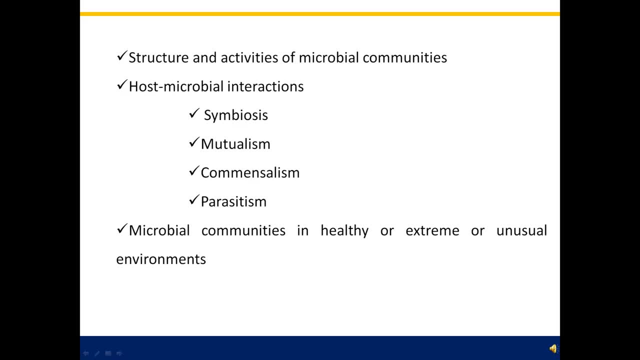 To the host, So they bring no benefit to the host. So, while the microorganisms are greatly benefited for the inhabited environment- So example is staphylococcus on skin, And next one is often parasitism- So parasitism, in this relationship one organism is benefited at the expense of its host. 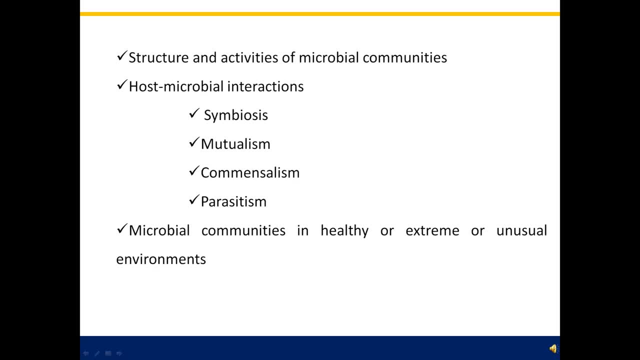 So the host will be affected And the microorganism will survive By getting an advantage of host. And next is often microbial communities in healthy or extreme or unusual environments. So we are going to study that. Okay, which microorganisms has been seen? is an terrestrial microorganisms or extremophiles or aquatic organisms and all? 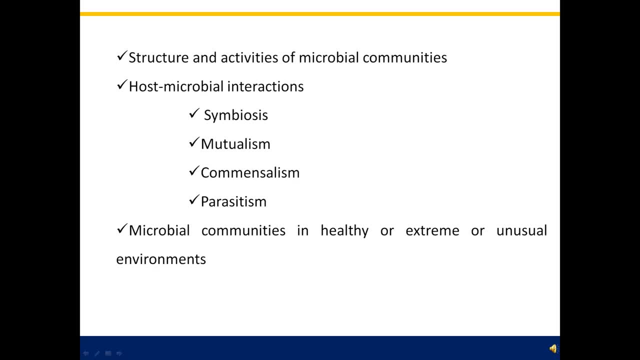 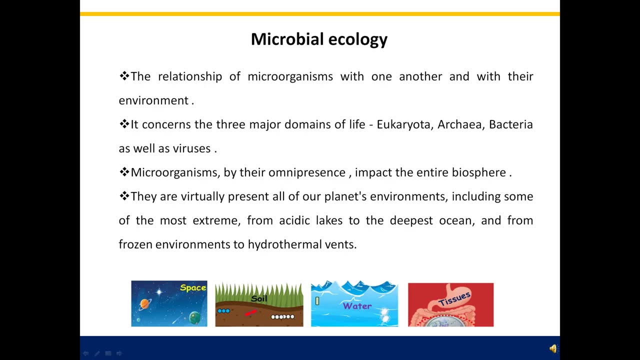 So these are the things which deals with an environmental microbiology, Microbial ecology. Microbial ecology deals with the relationship of microorganisms with one another and with their environment, So it is distributed into three major life domains, such as eukaryota, archaea and bacteria, as well as viruses. 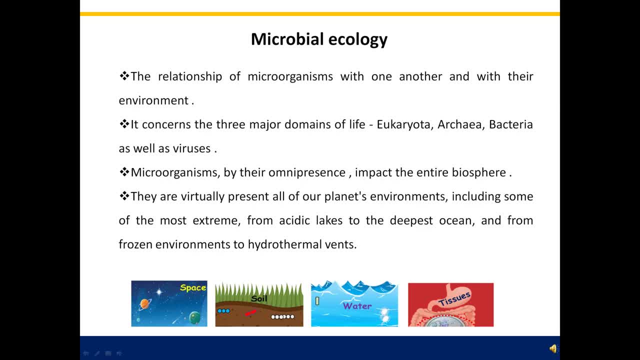 So, as we all know that these microorganisms are seen everywhere, So they are called as an omnipresent, Which in turn impact the entire biosphere. So this microbial life plays a primary role in regulating biogeochemical systems and virtually all of our planet's environments. 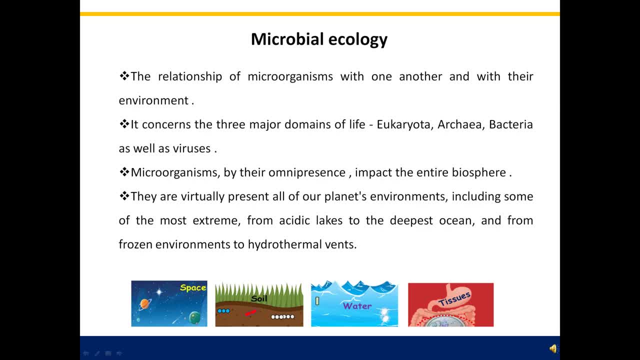 Including some of the most extreme, most frozen environments and acidic lakes, to hydrothermal vents at the bottom of the deepest oceans And some of the most familiar places, Such as human small interstates. So studying these microorganisms, the presence of these microorganisms at various conditions and various regions. 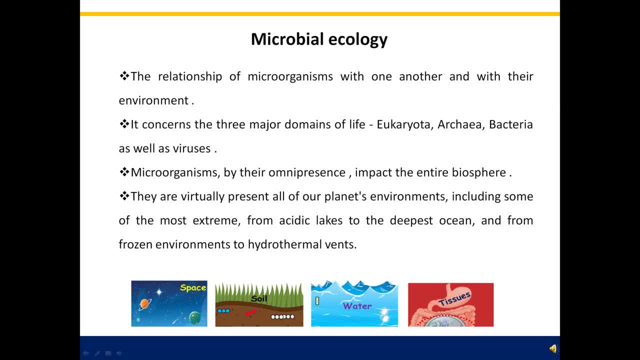 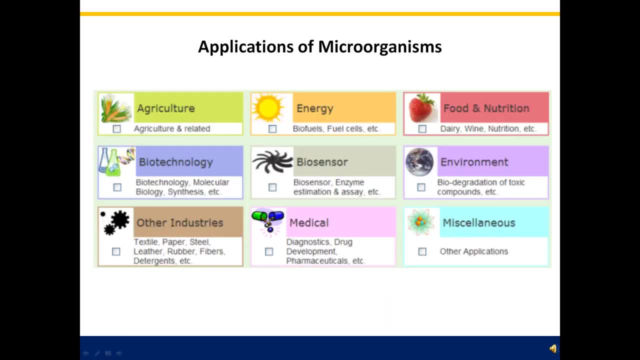 Or simply we can call it as of a microbial ecology, Or we are going to deal with a microbial diversity. So next, coming to the application of microorganisms. So as we know that these microorganisms are seen everywhere, So definitely they are having potential applications in every sectors. 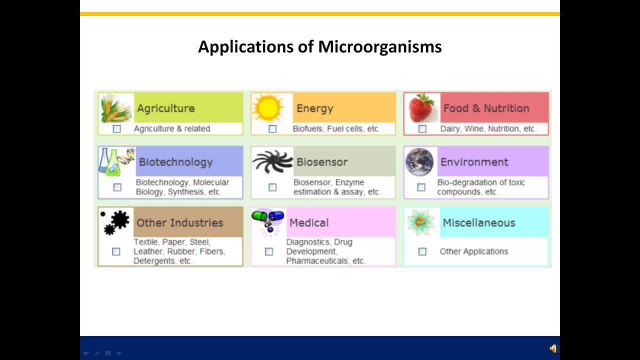 Like agriculture, in which it helps us to make and draft resistant plants- Pesticide resistant plants- So many- And the energy making and biofuels and fuel cells etc. And coming for food and nutrition applications. They have a vast range of applications, like in dairy products, wines, nutrition making and probiotics. 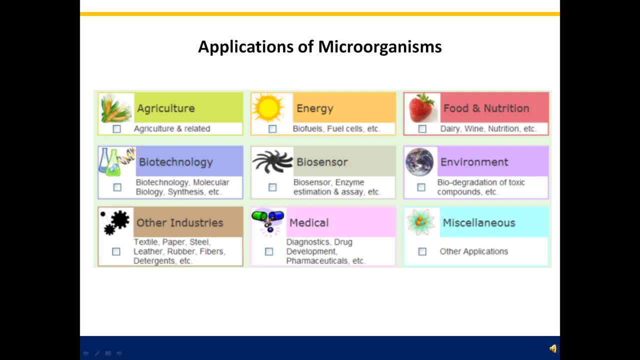 And coming for biotechnology applications. They have a major role in making synthetic antibiotics By using recombinant technologies And coming for biosensors. They help in making enzyme estimations and assay productions And coming for environmental applications like biodegradation of toxic compounds. 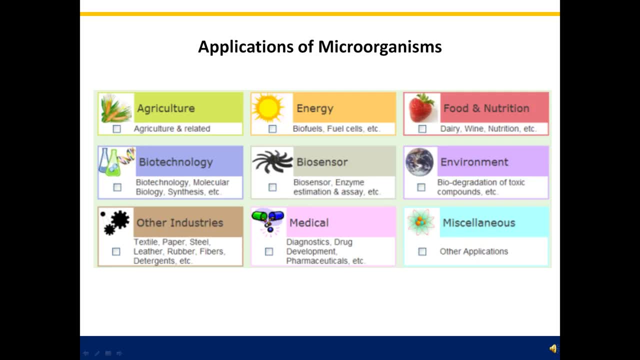 Like making xenobiotic compounds, Synthesis of xenobiotic degrading microorganisms, Like in superbug creations, And coming for other industry applications like paper industry, Steel, leather, textile, fiber, detergents, Say for like making an anti-corrosive steel products. 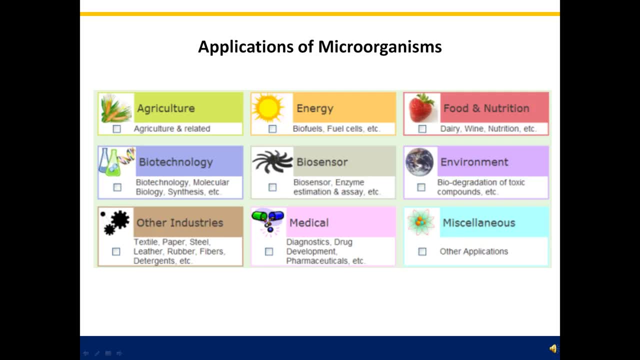 So where the microorganism helps To have a long lasting life for the steel, Stainless steels, That's called an anti-corrosive agents And, coming for a medical industry, So helps in making and diagnostic aids And making antibiotics. 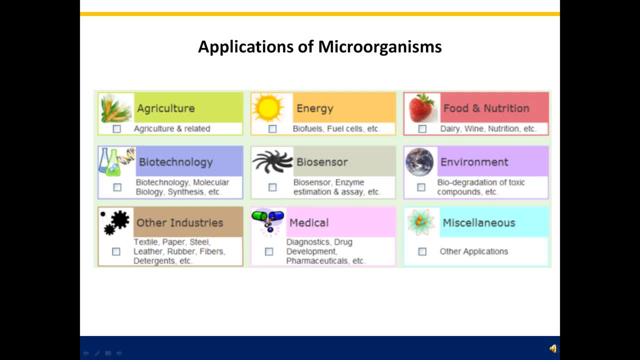 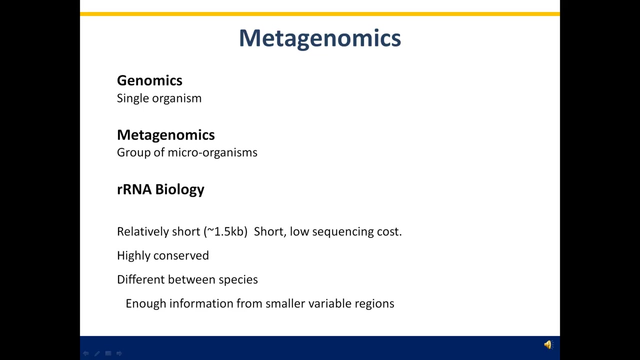 Like developing a new drugs. So it's having a vast measure of major applications Which helps to make the role of microorganisms are very essential As they have been seen everywhere in the nature. So next coming for the metagenomics, So of all the living organisms on the planet. 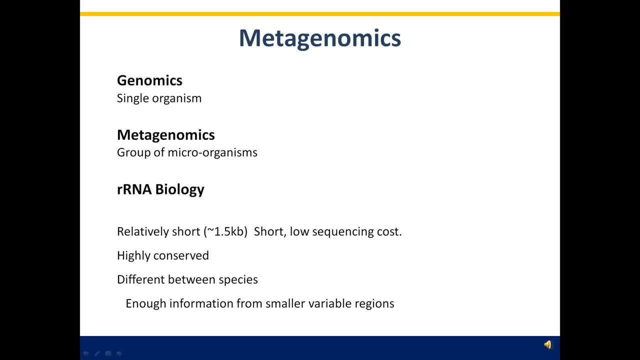 Microorganisms are the most numerically abundant and diverse in nature. So researchers have begun to understand their diversity, profiles, Metabolic functioning and potential economic values. So, in general speaking, in classical investigations to study the microorganism One has to culture and study the selected microbe in the lab. 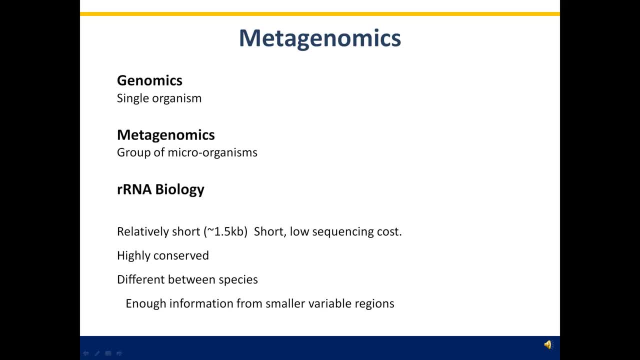 However, this approach can yield much information, Like saying: like so if you're going to deal with a single organism, Then it's simply called as of in genomics. So studying the genome of one single organism is called as in genomics, Whereas if you're going to deal with a group of microorganisms. 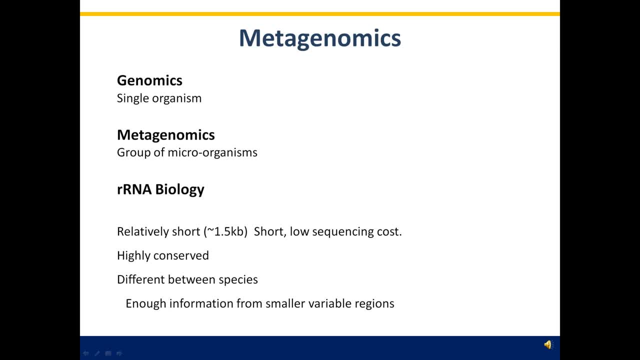 Then it's called as in metagenomics. And if you're going to study the microbial community Based on and analyzing the DNA within an environmental sample, Then it's called as in environmental genomics. So example includes profiling microbial population in water samples. 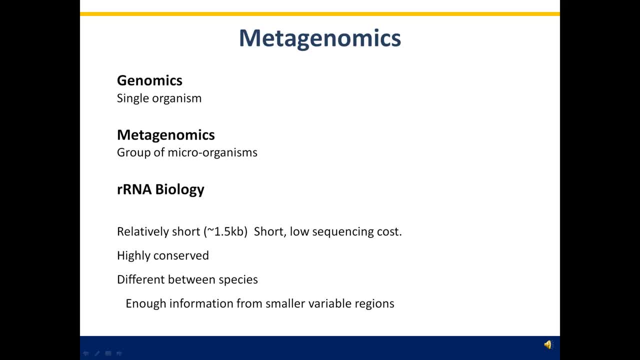 Taken from deep oceans or in soil, samples from human made environments Like active mineral mines, and environmental, micro, environmental, metagenomic study data Are used for agriculture, microbiome analysis, Ecology remediation and other biological investigations. So, coming for all this, So we need to know an RNA biology. 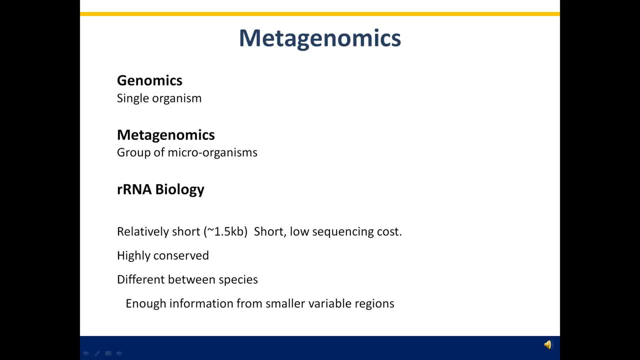 So which 16S rRNA is very important? So, as the 16S rRNA are relatively short, Which will be around 1.5 KB, and these are short And because of short sequence The sequencing cost is very low And this 16S rRNA are highly conserved. 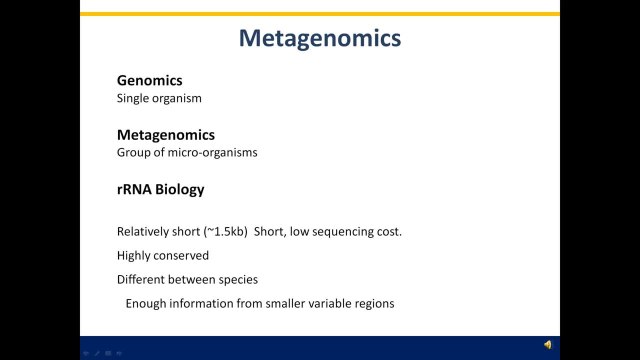 And definitely they are different between the species, So which makes an unique for each and every species, Though we cannot identify and species at 16S rRNA, But this is very helpful to differentiate the species And a small piece of information- A small variable region- is enough. 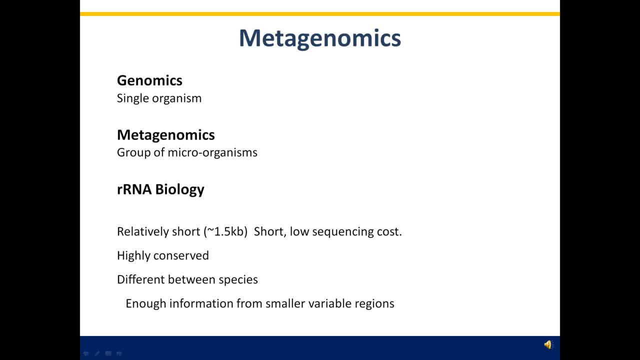 To have and much more informations. So, in general, this metagenomics deals with and sequencing A group of microorganisms And sequencing the 16S rRNA of a group of microorganisms By using a specific variable regions From the 16S rRNA region. 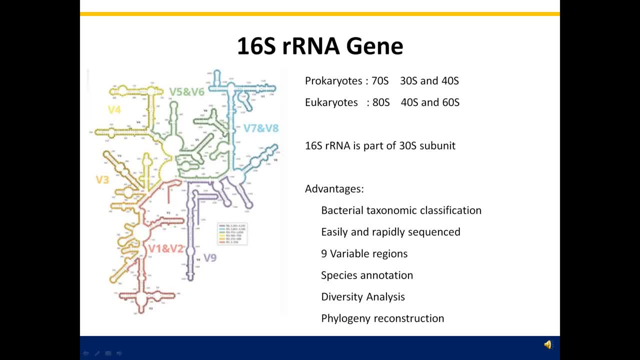 So next, coming to an 16S rRNA gene markers. So this 16S gene, This 16S rRNA genes, Are generally called, as often, gene markers. So in prokaryotes We have 70S ribosomes. 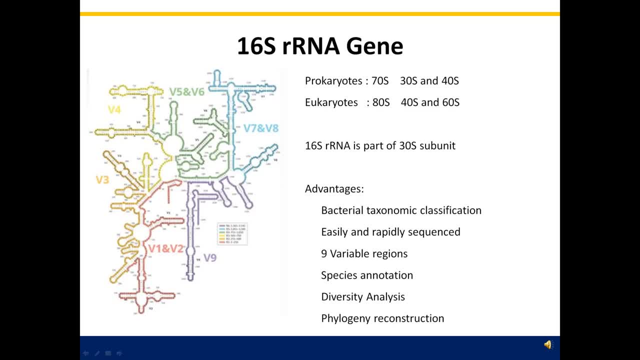 Made up of 2 subunits of 30S and 40S, While in eukaryotes We have 80S ribosomes Made up of 2 subunits of 40S and 60S. So coming to an prokaryotes. 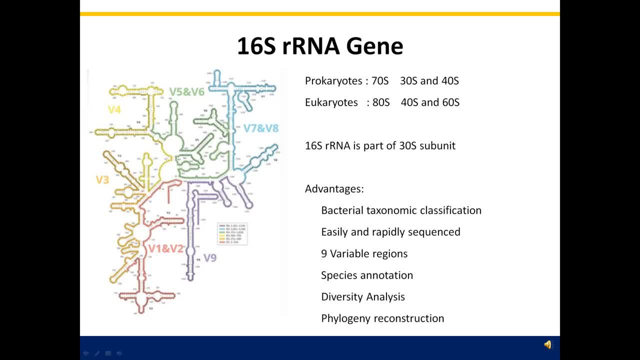 This 16S ribosomal RNA Is a component of 30S, small subunit of the prokaryotic ribosome That binds to the shine dalgerno sequence, Or simply we can call as often SD sequence. So the genes coding for this. 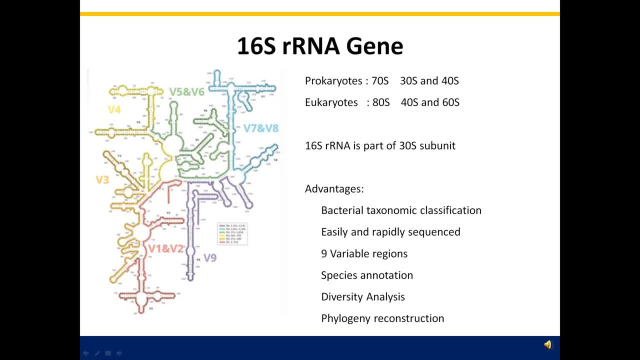 Are referred to as an 16S gene And are used in reconstructing phylogenesis. So it's due to the slow rate of evolution Of this regions in the genes. So this ribosomal RNAs Are classified into 16S, 23S and 40S. 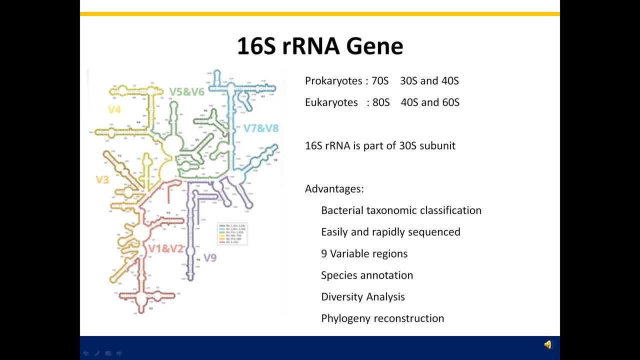 5S rRNA According to their sediment rates. So in general, This 16S rRNA has become standard Gene In bacterial taxonomic classification Because it is more easily and readily sequenced And contains enough phylogenetic information. 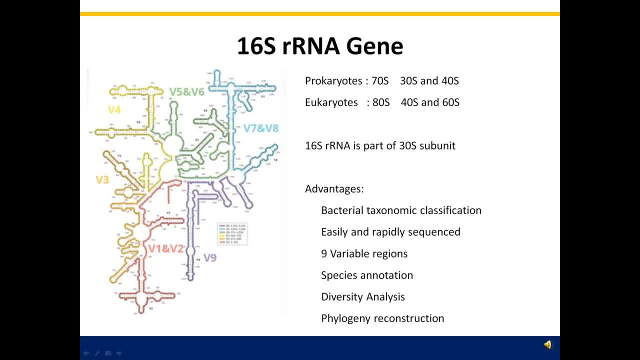 With short stretch of sequence. So this 16S rRNA gene consists of 9 variable regions, And these regions, The sequences of these regions, Are usually used for Species annotation, Phylogeny And diversity analysis. So these are the primer sets. 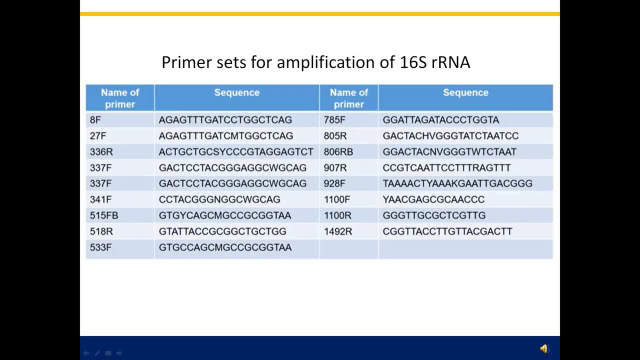 For amplification of 16S rRNA. So there are various commercially available primers For sequencing the 16S rRNA gene. In general, The whole length of 16S rRNA gene Is sequenced By using 27F. 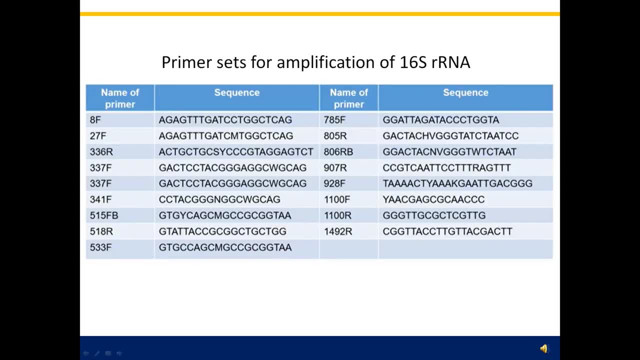 And 1492 reverse primer sets, While the other primers Are used to sequence By using various sequencing technologies Like Sangha sequencing Or Pacbio smart sequencing, Because different lengths of DNA Are sequenced By various sequencing technologies. 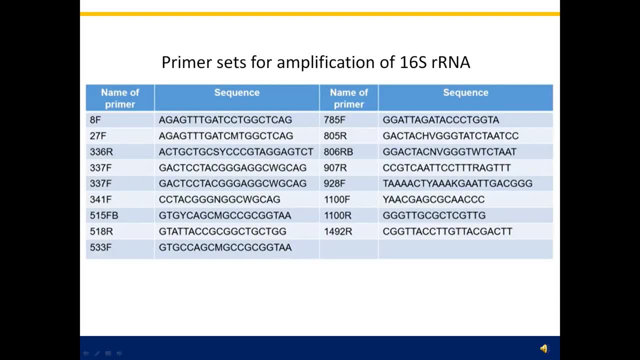 So one can use The suitable set of primers For their sequencing technologies. Say, for example, Most commonly The people used to prefer At V3, V4 regions Like 337F And 805R. So these are the most significantly. 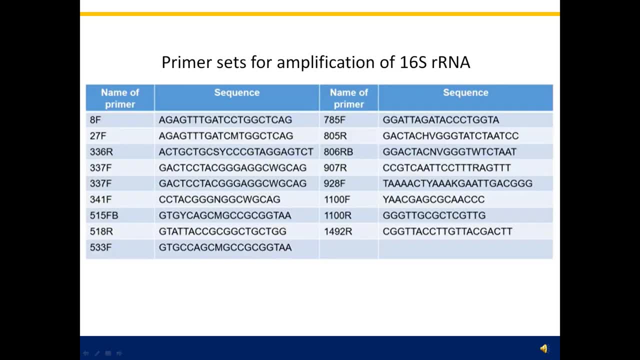 Used primers Or if you are going to sequence The whole length of your 16S rRNA, Then we can prefer, Like 27F And as we discussed, 27F And 1492 reverse Primer sets. 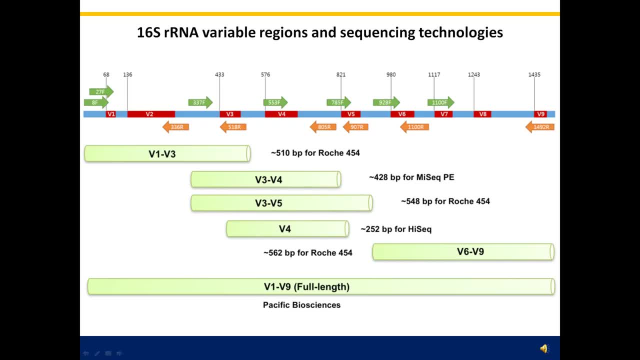 So next coming forth, These variable regions And sequencing techniques And sequencing technologies. So we have discussed That we have Different kinds of variable regions, Like V1 to V9 regions, And we have And specific primer sets For each and every specific region. 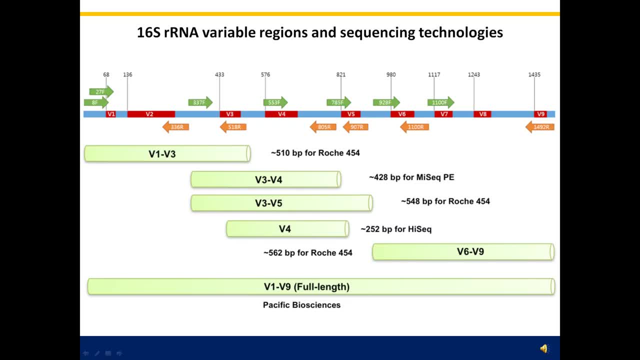 And if you, By looking into this picture, We can know that Which region Can be amplified By using Which kind of Sequencing technology, Say, for an example, And V1 to V3 region. So if you want to identify, 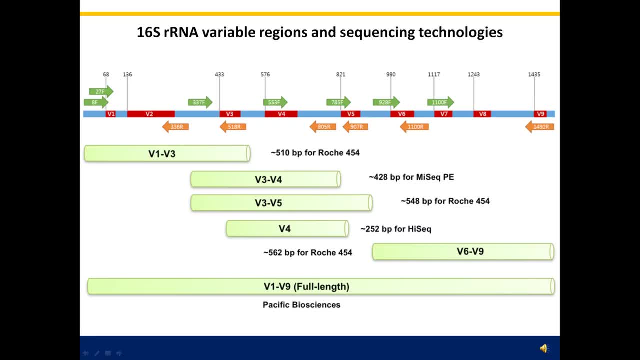 And V1 to V3 regions. It will be around 510 base pairs. So That will be. That can be sequenced By using Roche 454.. Sequencing missions And if you are going for V3, V4 regions: 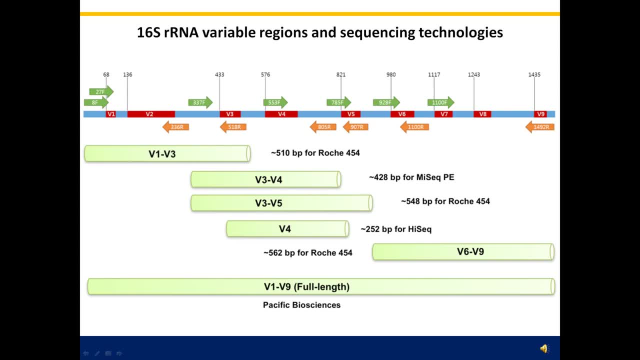 Will be. The targeted Site region Will be around 428 base pairs And this can be Used for An Illumina mysic Padent Sequencing. Again, V3- V5 regions: The region, The 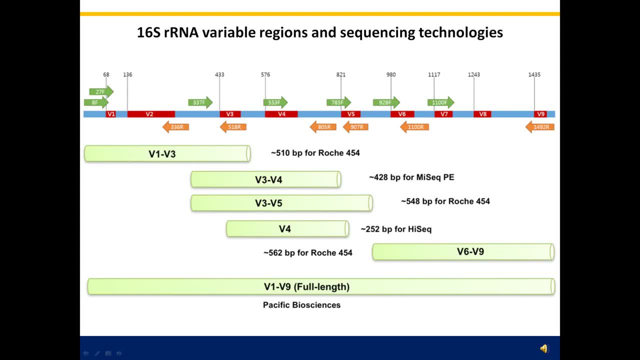 Targeted Length Will be of 548 base pairs Can be used by Use Sequenced by Using Roche 454.. And Just V4 region. We can Have A target region of 252 base pairs. 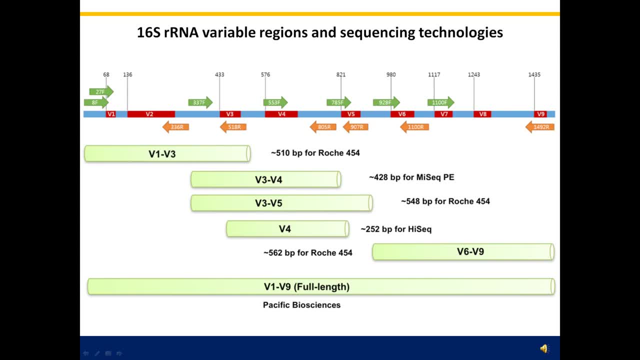 For Mysic And V6 V9 regions Is of 562 base pairs With Again Roche 454.. And If you want to Sequence The full Length Of the genome, Full. 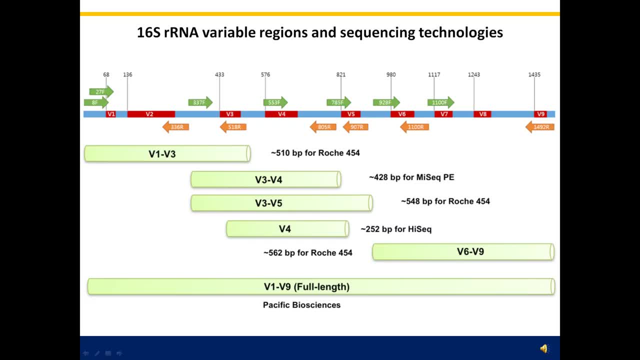 Length Of the System. So Like This, One Can Opt For What Kind Of Sequencing Which We Are Going To Perform And Which Region We Can. 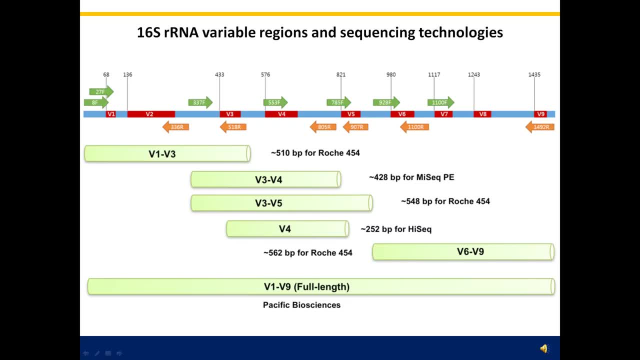 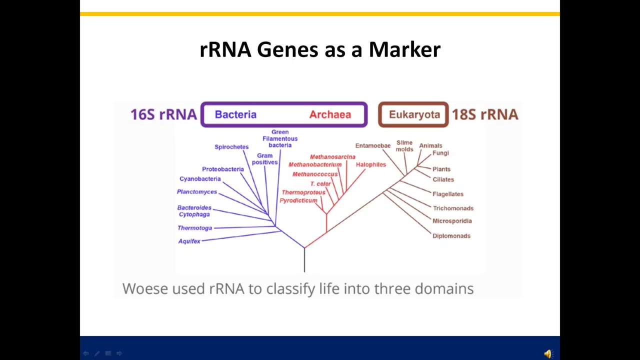 Target, And Mostly It Is A Bacterial Species Can Be Identified By Using This V3. And V4. Region. So Here We Are Going To. 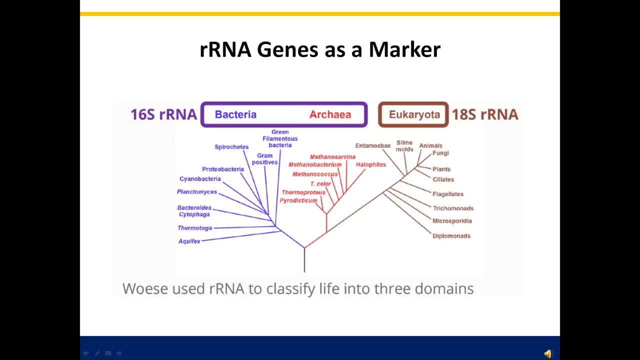 Say That RRNA Gene As A Marker. So We Have Presentation Of This. Three Kingdoms Of Life, So Where We Can Identify The Bacterial. 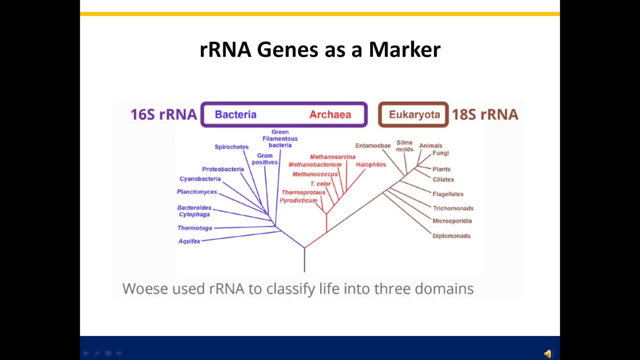 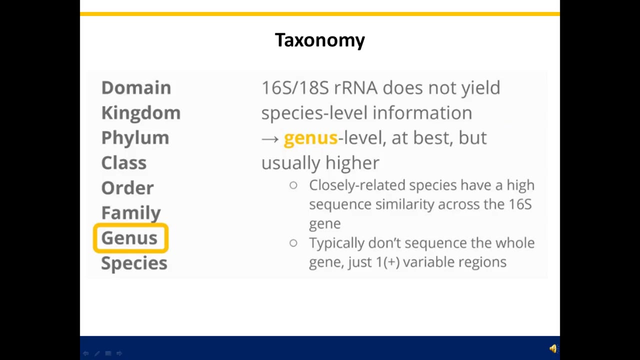 Archaeal Species By Using And The 16. As RRNA Genes, And While Eukaryotes Can Be Identified. So We Are Going To Find. 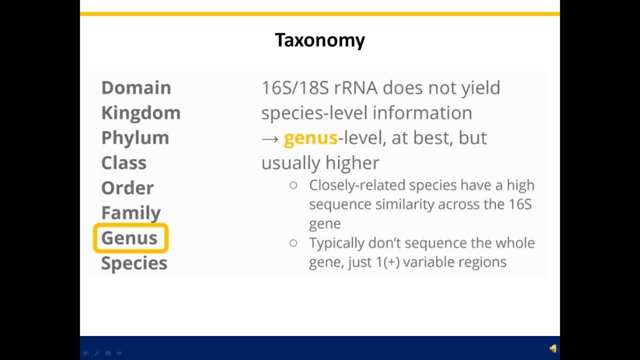 Out What Kind Of Bacteria Has Been Present In Our Source Samples Which We Have Isolated, So Say For An Example, Once We Identify The 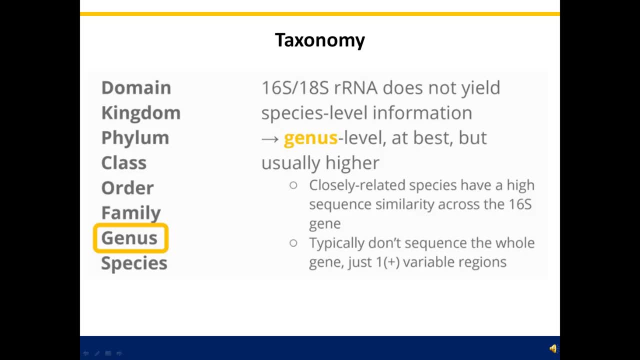 Bacteria In Our Kingdom It Belongs. So, In General, The Higher Level Of The Species Can The Higher Level Of The Organism Can Be. 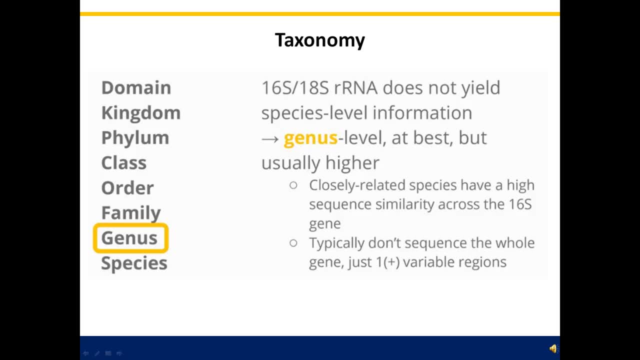 Easily Identified By The 16s And 18s, Or RNA, Are Very Important. So Genus Level Has Been Considered As Often Best, So This: 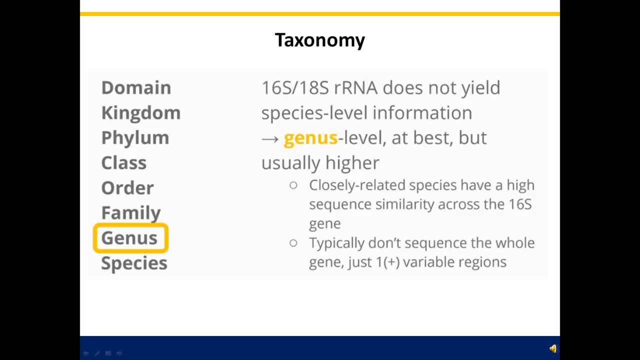 Can. The Organism Can Be Easily Identified, Closely Related But Specific Bacteria Belongs To, So I Remember That Once We Have An Sequencing. 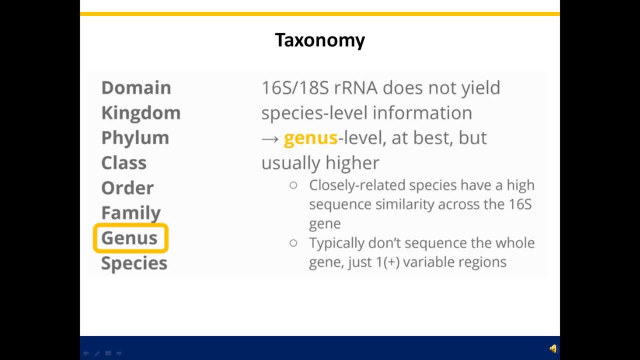 Of 16s RRNA, So We Are Going To Find Out To Which Genus This Particular, That So This Specific Bacteria, Has Been Identified. 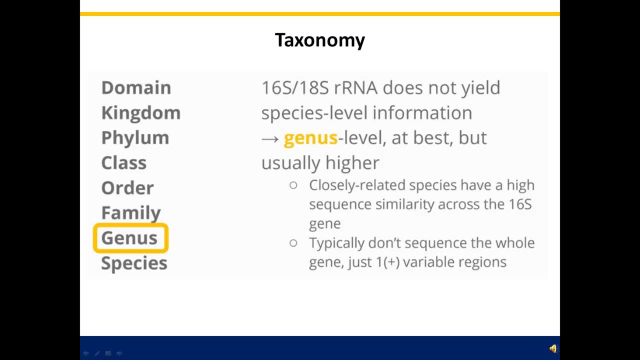 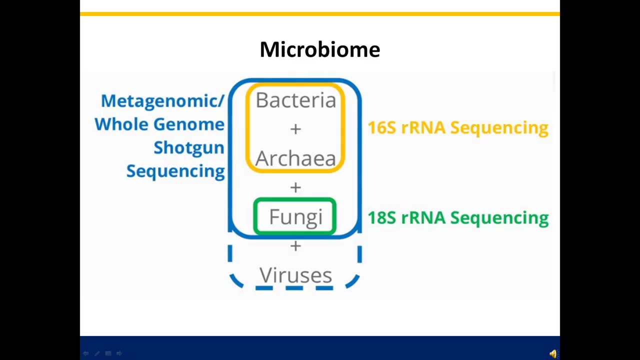 And To An Family Level Or Order Or Class, Phylum And Genus, And Mostly Sometimes We Can Say That This Is Our Whole Genome Shotgun. 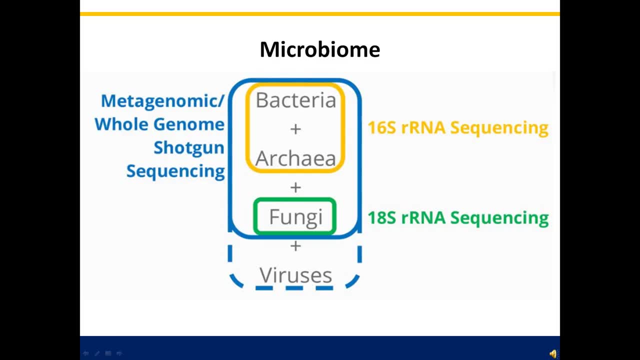 Sequencing, So Where We Are Going To Find Out What Are The Bacterias And What Are The Archeas Which Has Been Seen In. 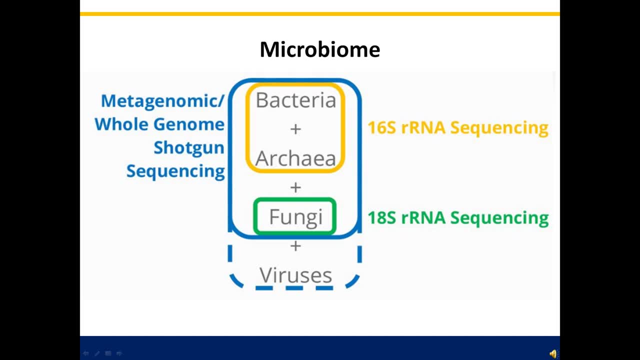 Our Samples With, And So If You Have Been Dealing With Only Within Bacteria And Archeal Sequences, The One Can Go For Only. 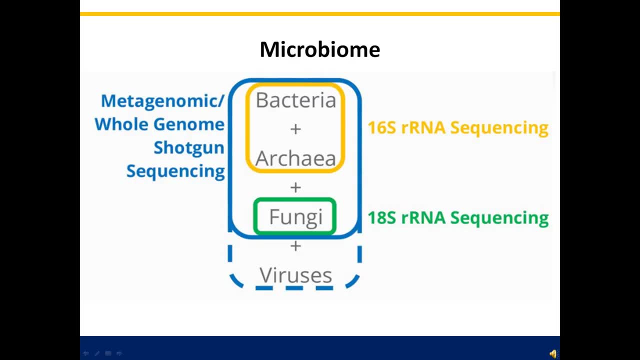 16S RNA Sequencing, Or If You Want To Find The Bacteria Which Has Been Present In The Whole Sample Site. So Simply, If You. 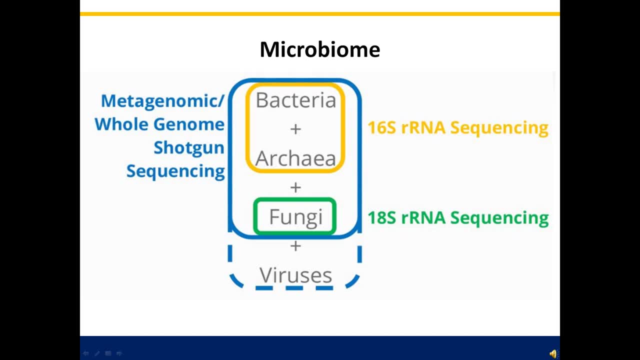 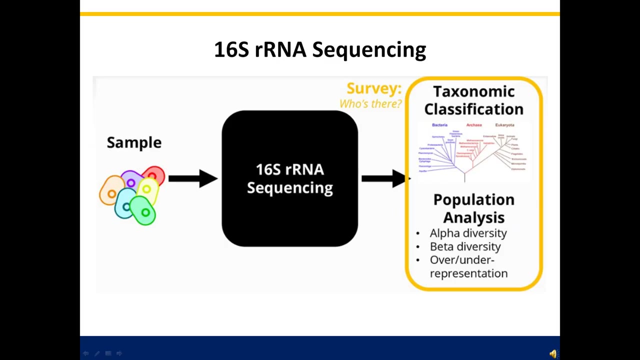 Are Going To Combine The Everything, Then We Are Going To Call It On The System, So, In General, To Perform This, Microbiome Studies, Or 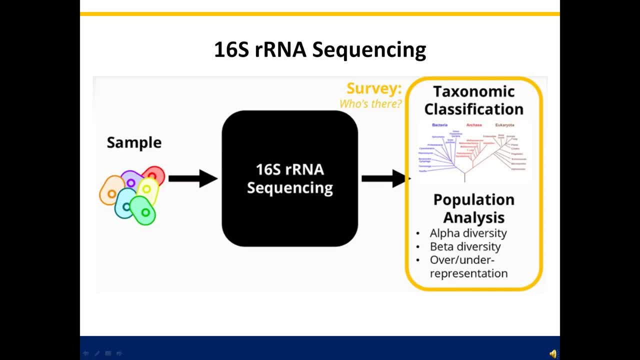 Metagenomics We We Are. We Have Been Heavily Dependent On 16S RNA Sequencing. So Once We Collect The Bacterial Regions, I'm 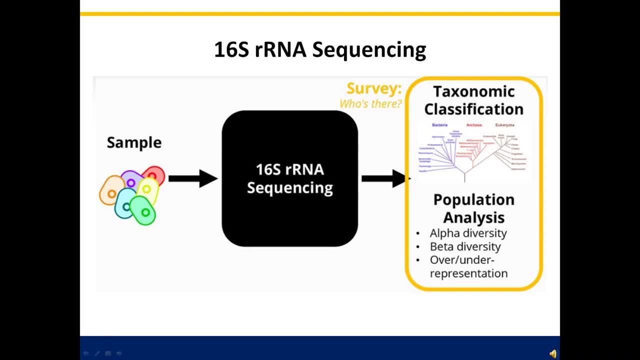 Going To Sequence That 16S RNA Sequencing And Then I'm Going To My Find Out What To Which Taxonomic Classification My Bacteria Belongs. 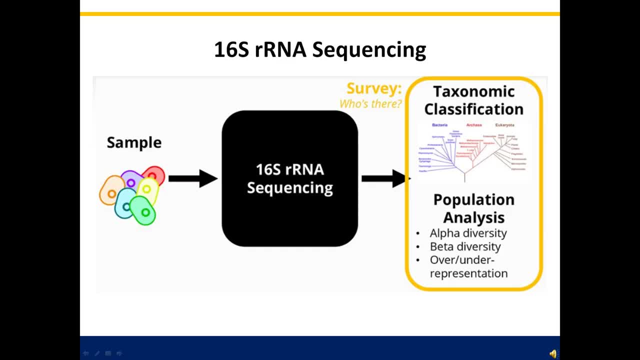 To. So You Can, Of Course, If You Are Going To Use An 16S RNA Sequencing, We Will Be Having Only A Bacterial Archaea. 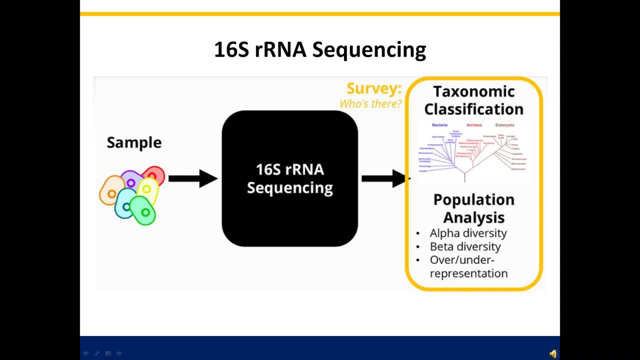 And Further We Are Going To Do. This Kind Of Survey Will Help Us To Know That Which Specific Community Or Which Is A Specific Phylum. 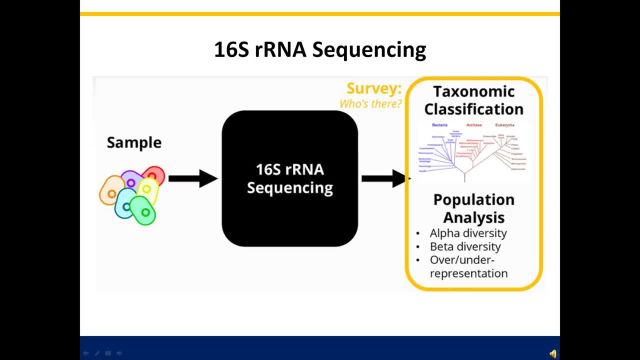 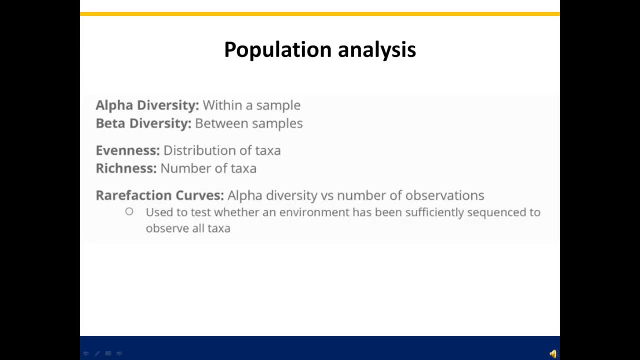 Is Very Essential For Maintaining The Plant's Health Or Growing. So, Coming For The Population Analysis, This Is The Most Important Analysis From Our Microbiome. 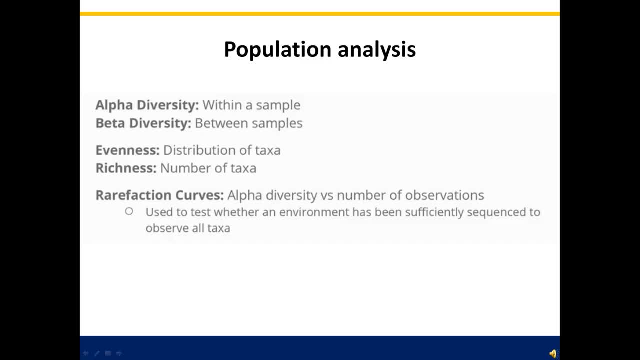 Point Of View, Or From Metagenomics Point Of View. So The Two Kinds Of The Distribution Of Taxa. So How? The Distribution Of The 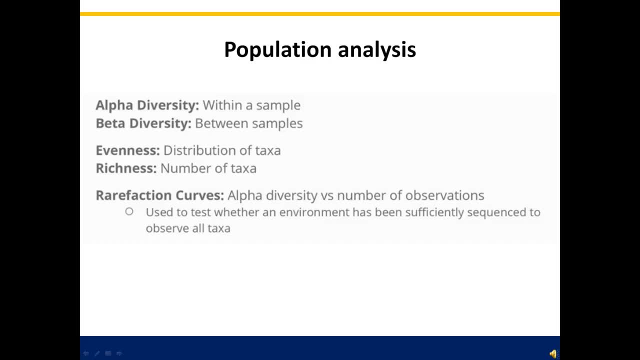 Taxa Has Been Present, And Richness- How Many Taxas Has Been Present, And Rarification Curves. So Which Says That This Sample Is Considered. 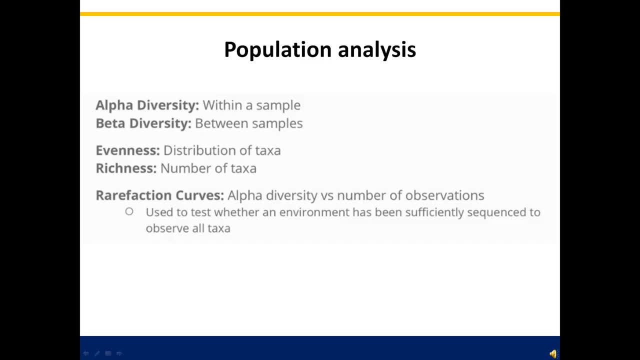 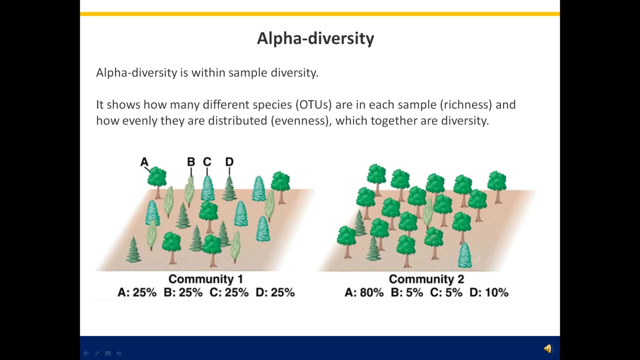 Or Not For My Further Analysis. So, Coming To This Population Analysis, It's Very Important To Identify An Alpha Diversity And Beta Diversity And Sometimes, 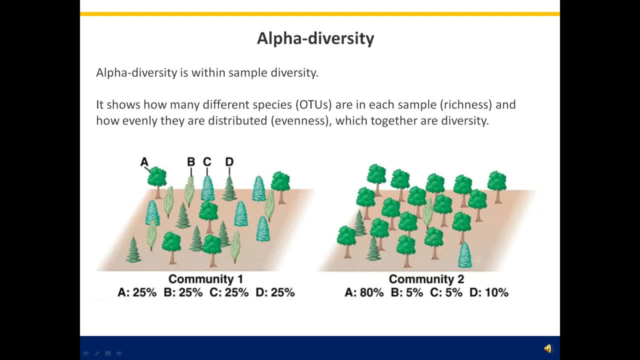 Alpha Diversity Is Within Sample Diversity, So It Shows How Many Different Species Of Water Use, Or In Each Sample That's Called As A Richness. 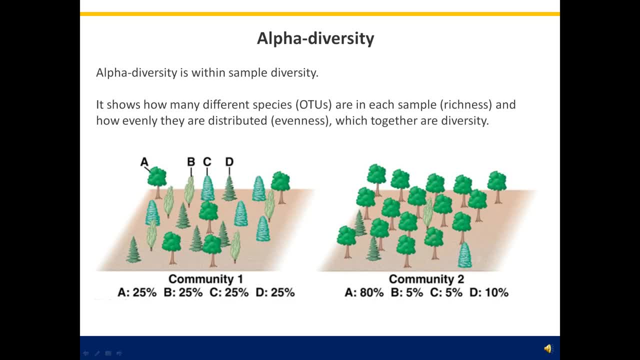 And How Evenly They See The Community One Is Having And Same Richness Of Four Tree Species, So Where You Can See That The Community 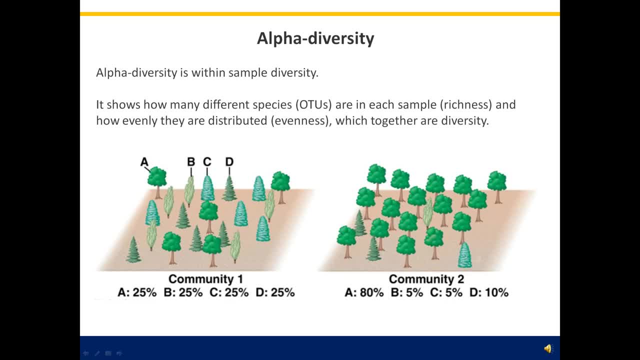 One Where The A, B And C, D Is Higher, Like 80%, And B Is Of 5%, C Is Of 5% And D Is 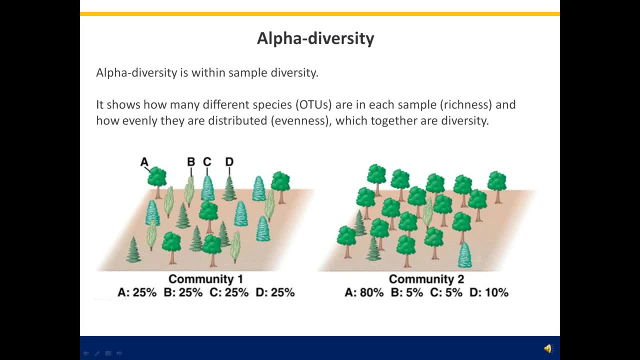 Of 10%. So This Says That Community One Is More Diverse Than Community Two. Is Dominated By Three Species. Community Two Is Dominated By 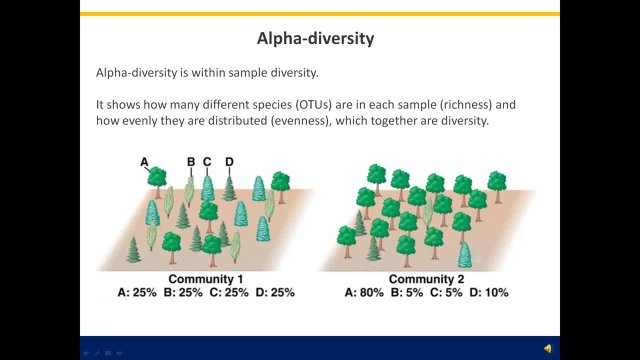 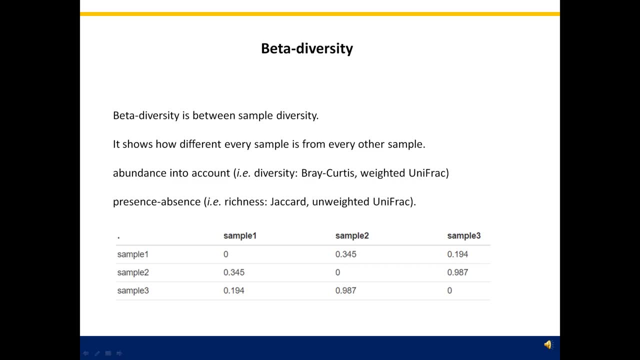 And Three Species. This Makes Community One More Diverse Than Community Two. So Next, Coming To The Beta, Diversity Analysis Are Made Up Of And: 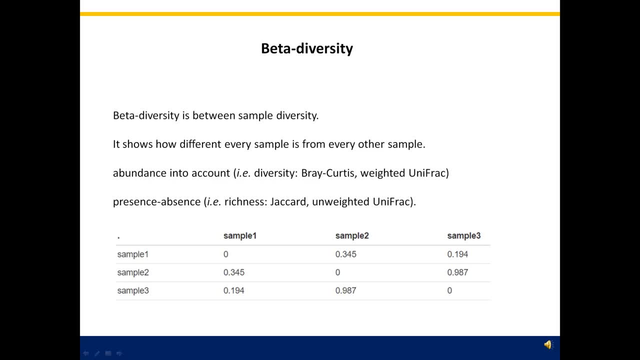 Completely Made Up Of Numbers So You Can Say That When Calculating Beta, Diversity Few, Diversity Analysis, Calculations Like Break Ortiz And Wade Jackered. 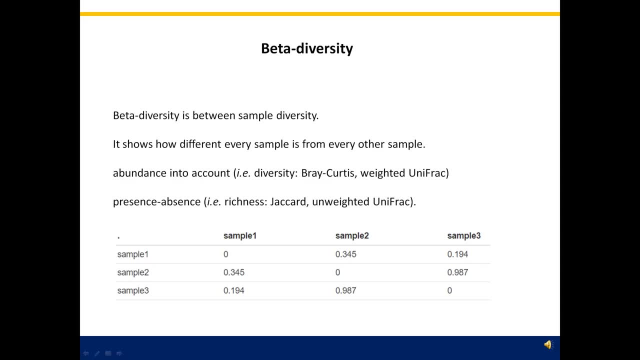 And Unweighted Unifrag Methods, The Presence Or Absence Of An Species Will Be Considered. See In This Illustration. You Can See That The 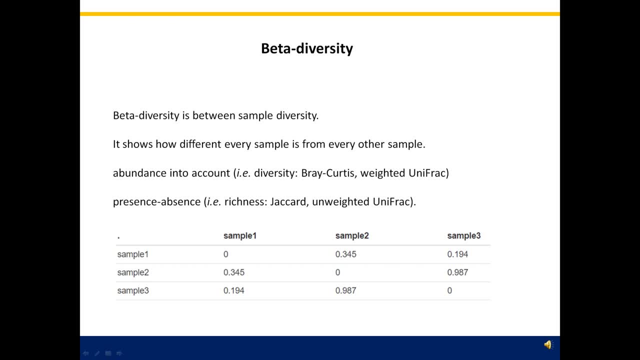 Table. So How? What Is Significant Difference? And So We Have To Perform An Statistical Analysis And We Can Say That Whether There Is Any Statistical 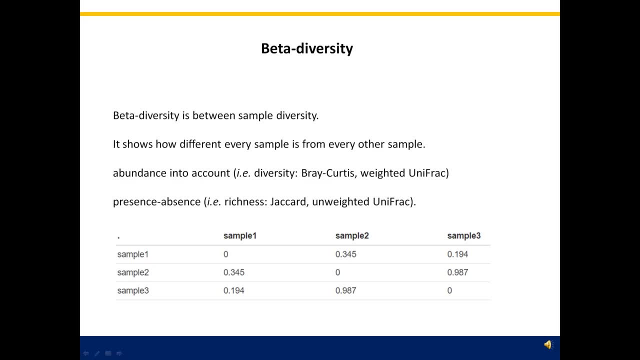 Significant Difference Between The Samples Or Not. So We Can See How Different Samples From Each Other Is By Using An NMDS Method. It's Called. 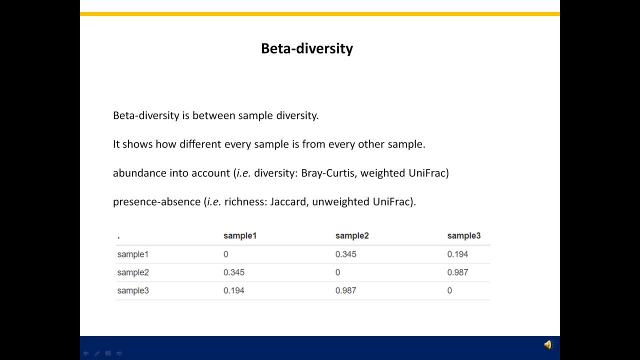 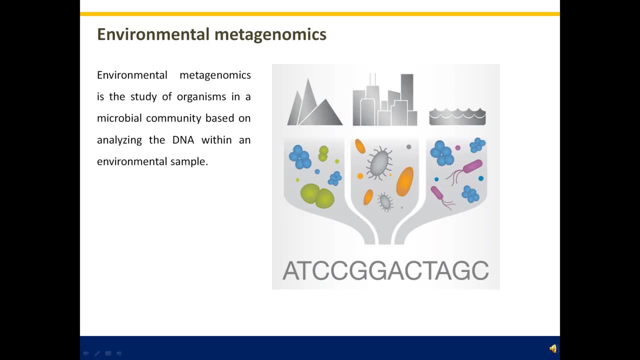 As Of A Non-metric Multi-dimensional Scaling, And This Method Will Be Simple. So An Meta Genomics Is A Study Of Organisms In A 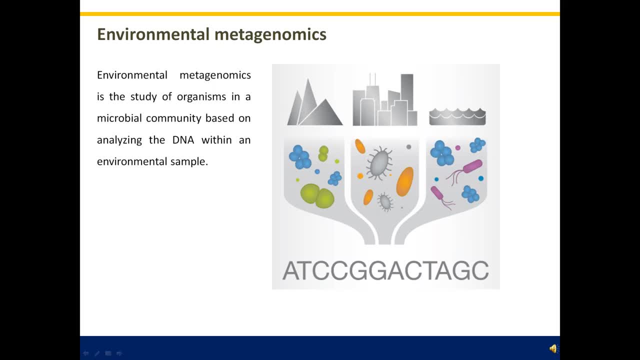 Microbial Community Based On Analyzing The Dna Within An Environmental Sample. So The Examples Includes Like Profiling And Some Marine Sources, So These Environmental 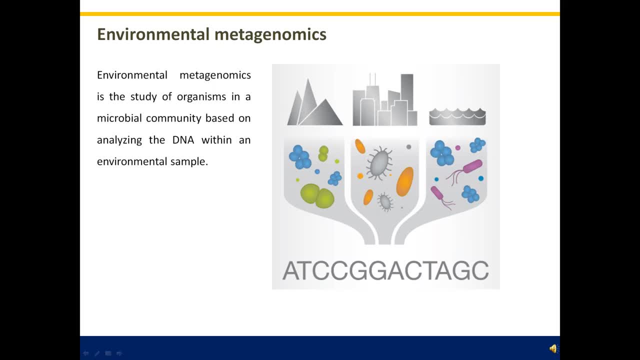 Meta Genomic Studies Are Used For Agriculture, Microbiome Analysis, Ecological Remediations And Other Biological Investigations. So, In General, With The Ability To Combine 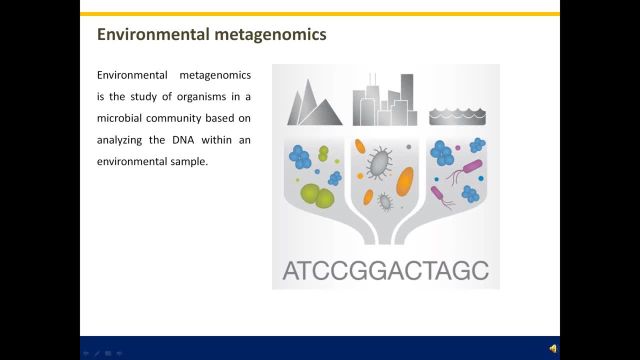 Many Microbes In The Environment It Is Expensive To Identify Using Other Methods, So Such As Most Microbes Present In The Environment Are Unculturable. 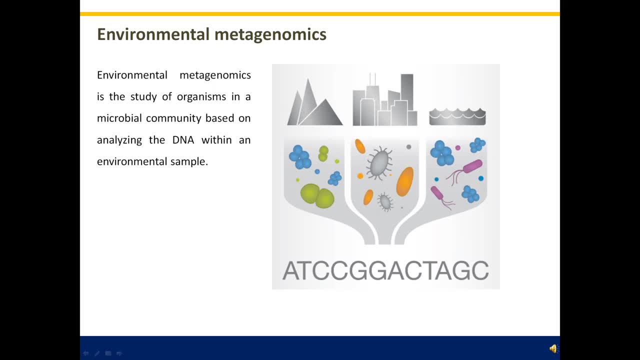 While Using Currently Available Media Methodologies, Have Gained An Attention. So At This Point, The Development Of High Throughput Sequencing Technologies Has Dramatically 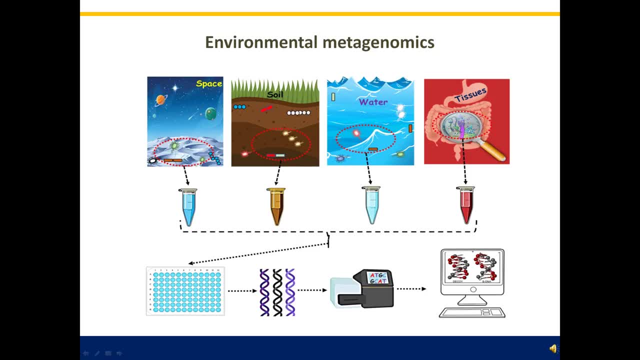 Advanced To Conduct The Analysis Of Microbial Species, Diversity And Their Functioning, And Researchers Provided The Researchers With The Capacity To Profile Entire Microbial. 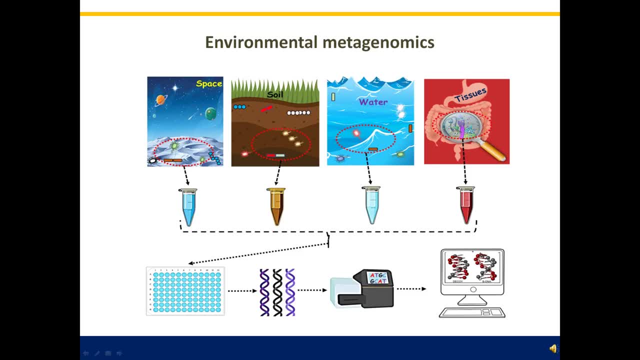 Communities From Complex Samples And Discover New Organisms And Explore The Dynamic Nature Of Microbial Population Under Changing Analysis Of Microbial Whole Genome Sequencing. 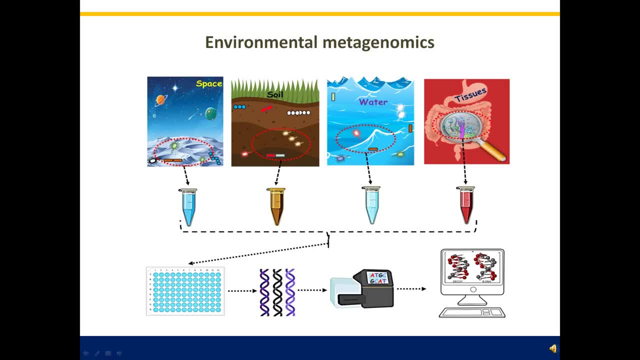 And Denova Assembly And Microbial Meta Transcriptomics. So In General, Once The Researchers Can Obtain The Millions Of Sequence Reads From The Selected Genomes. 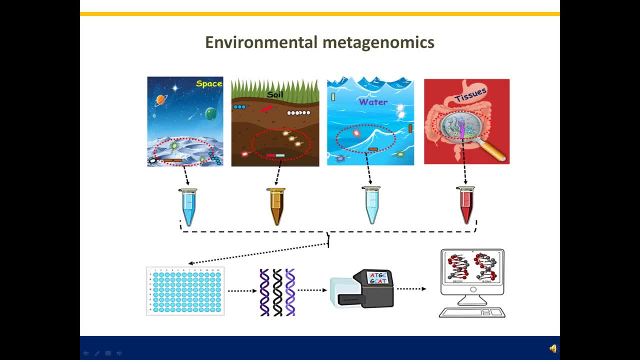 Which The Overlapping Sequence Reads Are Paid Much Attention. So, However, This Assembly Stuff Is Very Challenging, Because The Sequence Reads Are Generally Quite. 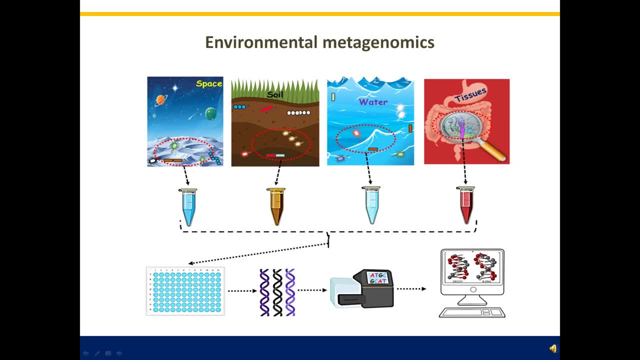 Small And Genomes. Often In Advanced Assembly Tools One Can Use And Reference Genome Sequences And Follow The Methods, And One Can Annotate The 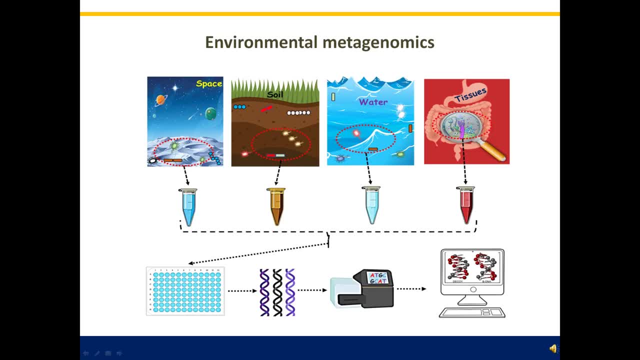 Genome. However, This Genome Annotation Is A Process Of Identifying The Genomes Are From And Basic Enrollments Like Soil Are. They Can Study The 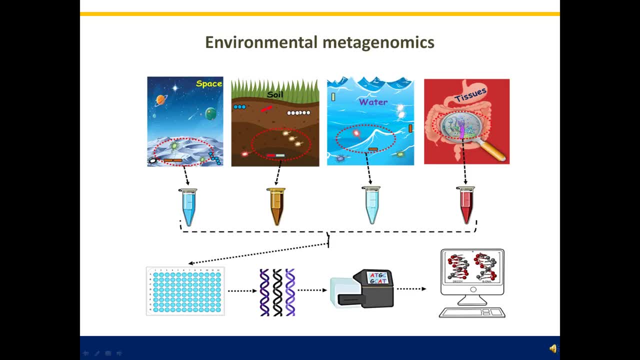 Samples From Water Study, The Samples From Human Tissues And Space. So Once The Samples Has Been Collected, The Librableries Will Be Prepared. 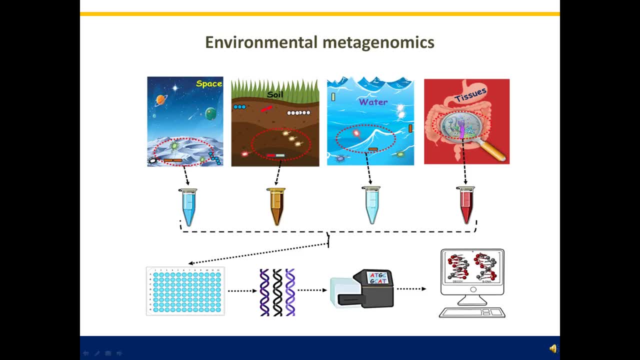 And This Libraries Will Be Taken For, And Sequencing Technologies Like. What are The Technologies analysis like which we have discussed in 16-inch RNA sequencing? like once the sequencing has been done, we are going for an survey to find out what kind of bacteria has been present. 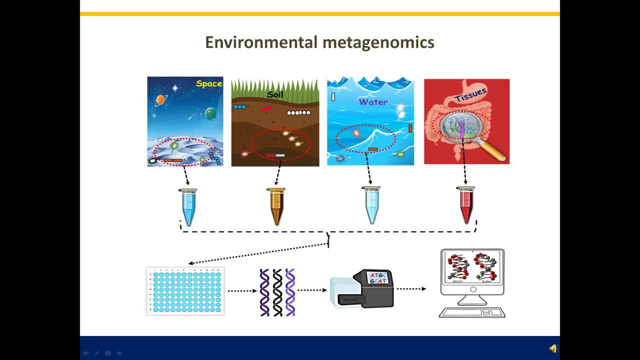 what other bacteria has been present. and then we are going to further do an taxonomical classification of that OTUs and we are going to say that we are going to study the population analysis like alpha beta analysis. so these are the various advantages of performing an. 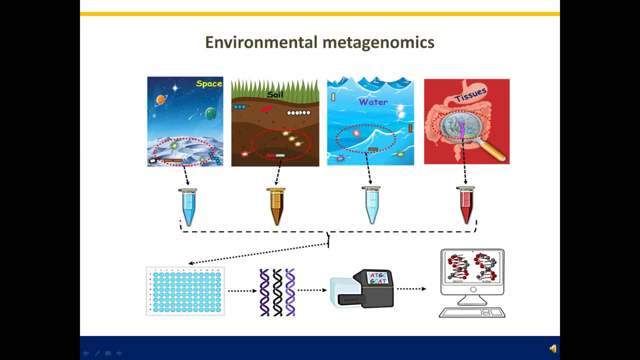 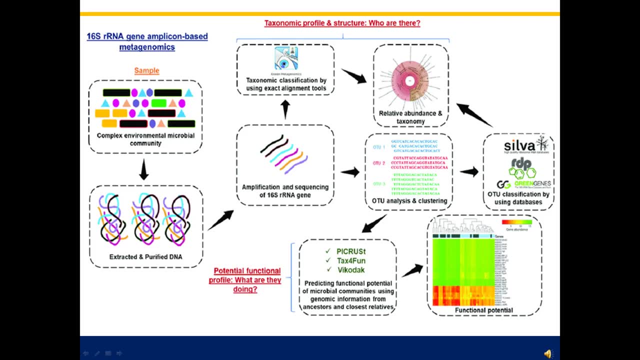 environmental meta genomics. so, coming to the most important sequencing technology in meta genomics, it's an 16-inch rRNA gene amplicon based meta genomics. so we are going to perform this to find out the taxonomic profiles and structures so that we can know. 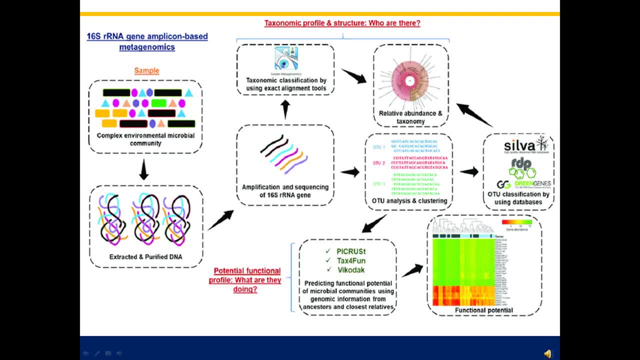 what bacteria are present and what they are doing actually. so here this follows and simple basic steps like collecting the samples, so the samples can be from an complex environmental microbial community. so once the samples has been collected, so we are going to extract and purify the DNA and this extract and purify DNA will be taken for an amplification, that's. 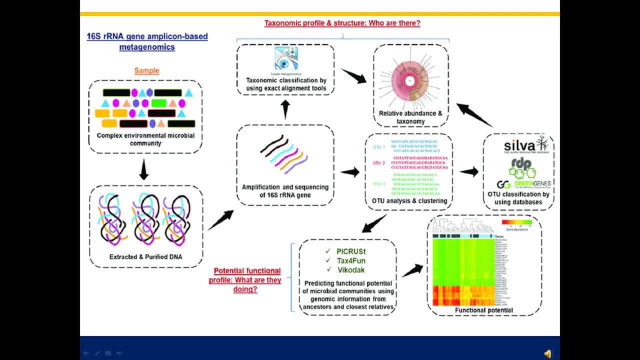 called SFN library preparation and after amplification and we are going to perform and sequencing analysis, sequencing um, 16-inch rRNA sequencing, say, for an example, here we can use an v3 before regions to primers to amplify. and then we are going to follow and my sequencing technology and once we get 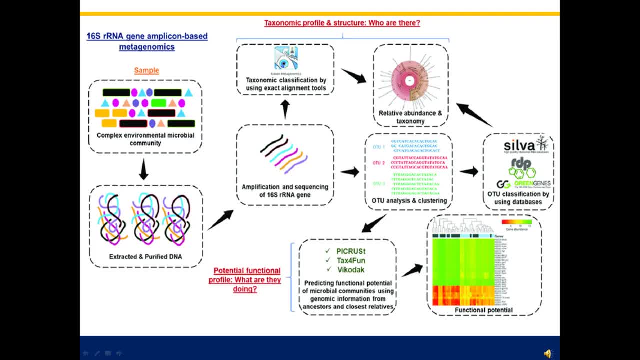 an sequencing reads. so those reads will be further processed, like in pre-processing steps like filtering what are the low, poor quality regions, filtering those stuff, and making and removing the camera camera regions, genes. So once it has been done so we will be getting an OTU. the reads will be considered as: 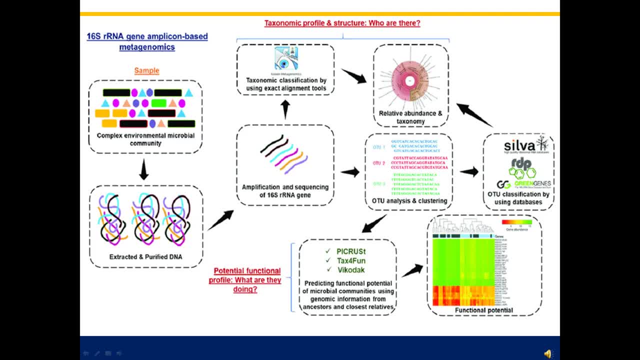 an OTU. So we are going to cluster that OTU and we are going to analyze that. So that's called as of an OTU analyze and clustering. And once it has been, what are you clustering and analysis has been done, we are going to refer that to an reference genome databases like for classification. 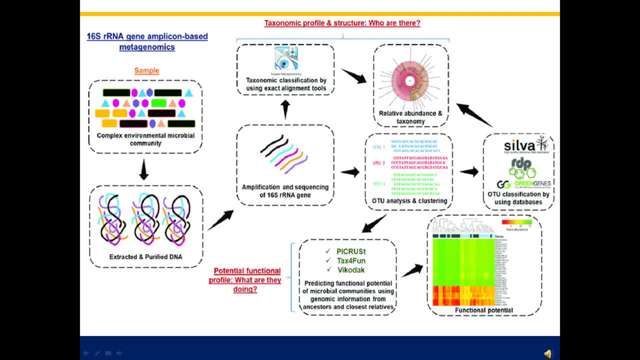 of this OTU by using and reference databases like silver, RDP and green genes database and easy taxon database. So once we classify the OTUs, so then we are going to check for its relative abundance and to which classification it belongs. So this relative abundance will give you an 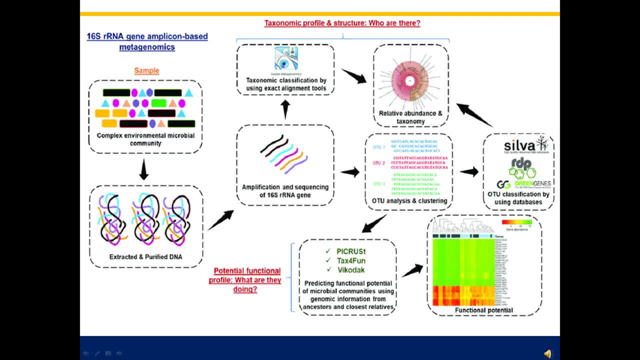 clear idea that. who is there present in the taxonomy? So what's the role? So which community is highly I mean, which phylum or which kingdom, which phylum or which genus is highly abundant and which is low abundant? So that's the one way of doing an relative abundance, or by going through. and what? 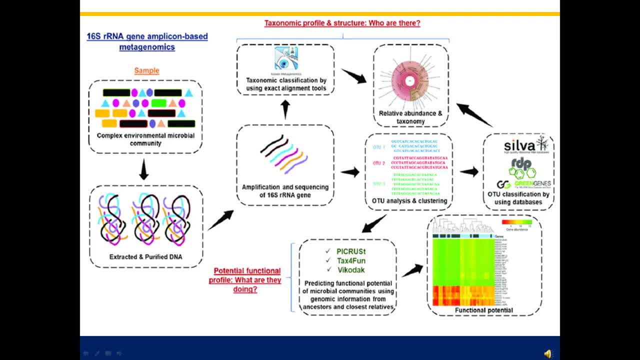 you analysis and clustering, or directly we can say that it's an taxonomy classification by using an extract. alignment tools like one can do with blast, and it's a tedious process where but the simple steps, like once the amplification is sequencing of 16th RNA gene- has been done, we can go for an OTU analysis and clustering and from there we are going. we can go for an OTU classification by using an reference database and then we are going for an relative abundance and to give an taxonomy classification. 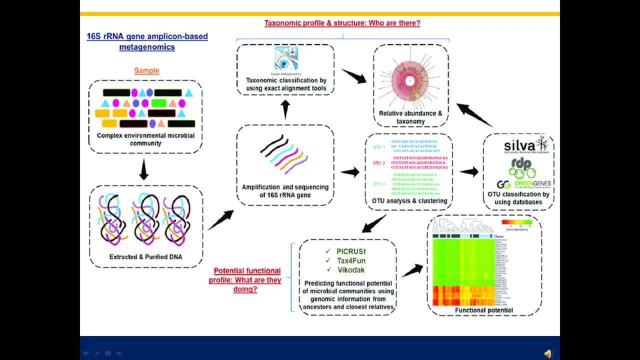 So this can be done with an and a chime 2 pipeline. So which we're going to discuss briefly, So how the pipeline works like, and once we have an OTU analysis and clustering, we can go for functional predictions, like we can identify the potential. 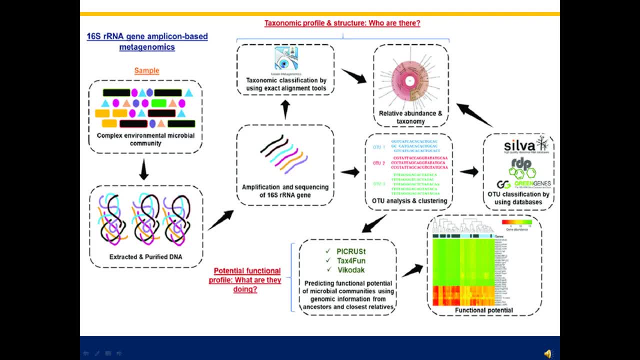 functions of a particular community and what actually they are doing. So for this we are going to use and different kinds of tools like pickress tax for fun We could act. So these are the tools which has been used for predicting functional functions of potential microbial communities. by using the genomic informations from ancestors and closely relative new, closer closest to Latius, One can make an functional potential. one can predict and functions and 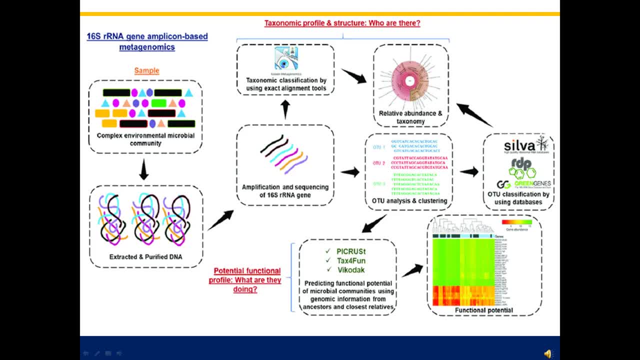 that can be represented as of an heat maps. so this all about the 16s rrna pipeline. so gene, gene application for metagenomes. so these are the steps which we are going to perform in our in the course of fourth session, with an hands-on training within some simple microbiome data sets. 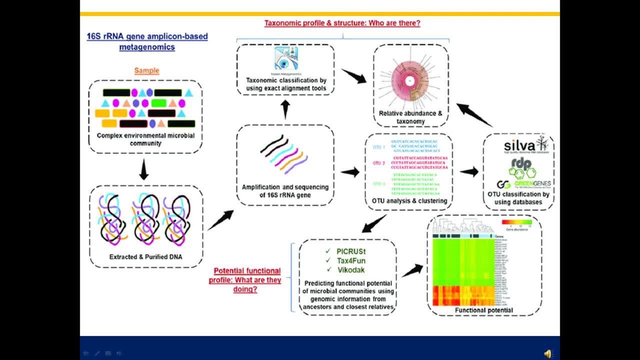 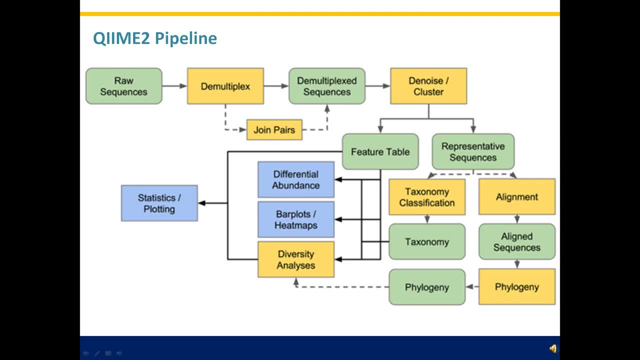 so this is all about our taxonomic profiling, so how we are going to perform. so this is the time to pipeline so, which we are going to discuss more detail when we are going for the further lectures. so here i just want to outline you what we are going to do here and this: 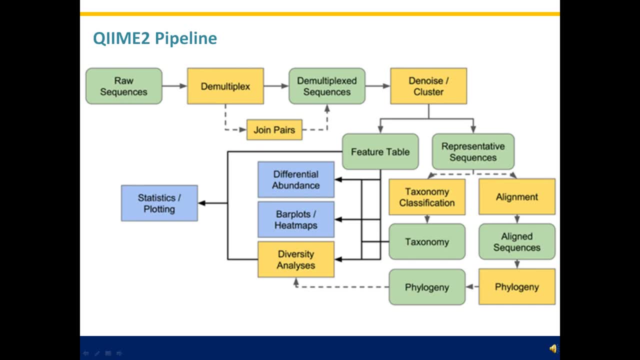 is what. this is the basic pipeline which we are going to use for all any kind of a microbiome or metagenomic data set. so once we get an raw sequences from our ngs technologies, so this, usually these sequences will be given with an barcodes so we have to demultiplex, so those are called as an multiplex sequences. so once we 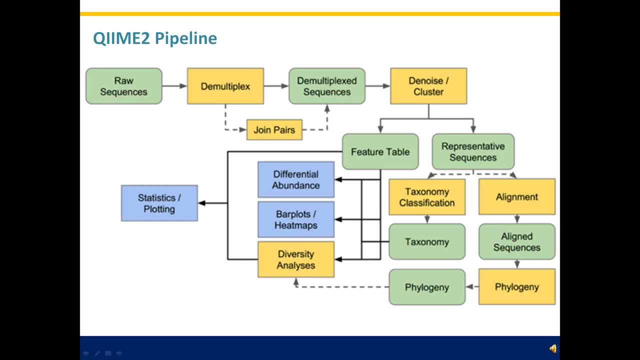 receive and raw sequences, we need to demultiplex it and we need to find whether it's an single end sequencing or paid end sequencing. so if it is unpaid and sequencing, join the pairs and then demultiplex the sequences. and once it has been demultiplexed, so we are going to denoise at the 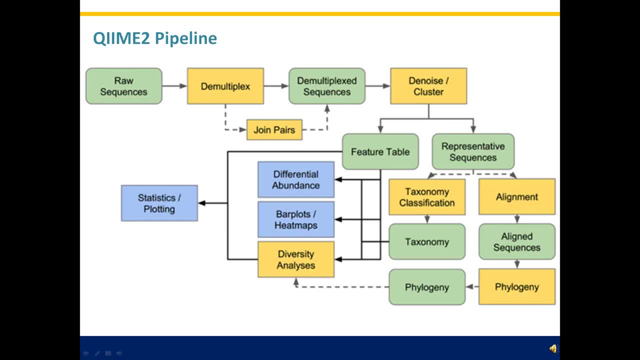 clustering. so this denoise is nothing is just like removing, filtering, the poor quality reads and any errors, and removing the chimera sequences and all. so this can be done by using and two different kinds of an algorithms like dada2 or a dblr. so once it's been 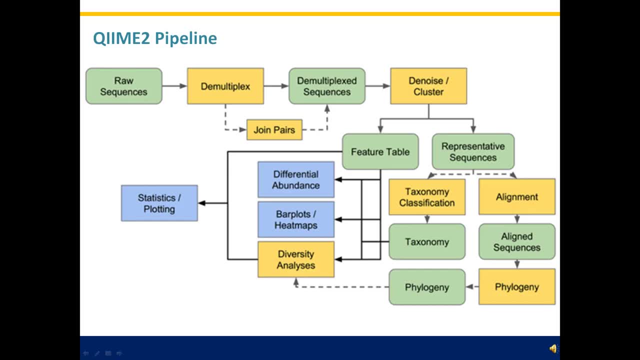 done. we are going to cluster our uh, what to use. so once the what use has been clustered, so we will be having an two kinds of an outputs: one will be in future table and one will be an representative sequences, so once we get. and future table, and one will be an representative sequences, so once we get. 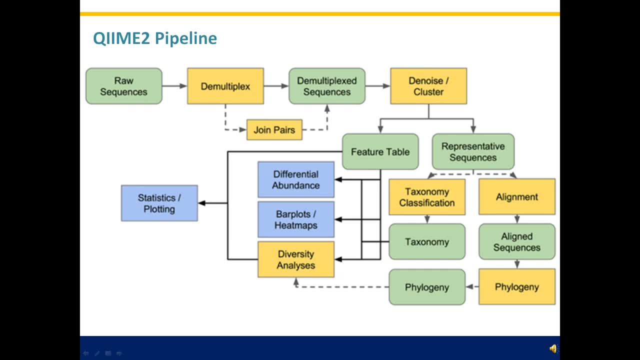 the future table. one can go for a statistical analysis or one can plot, so saying that what is the differential abundance, and bar plots are heat maps- or one can perform their analysis by diversity analysis, like alpha, beta diversities analysis, and then, with the help of an representative sequences, one can go for and building and phylogenetic tree by using uh, the. 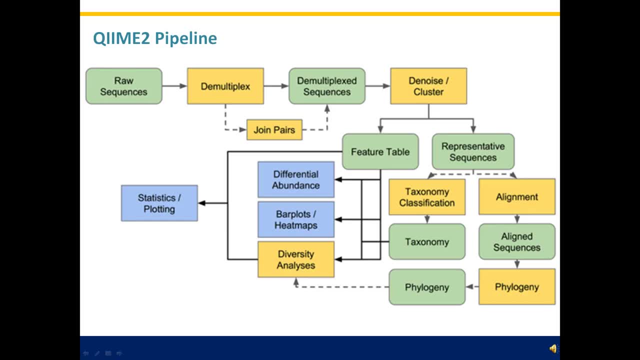 alignment methods by using an aligned sequences. so both the trees and unrooted trees can be built by using the phylogeny option and on another hand the taxonomic classification can be done, so saying the saying from kingdom to the species level. so most of the cases, the or it's an. 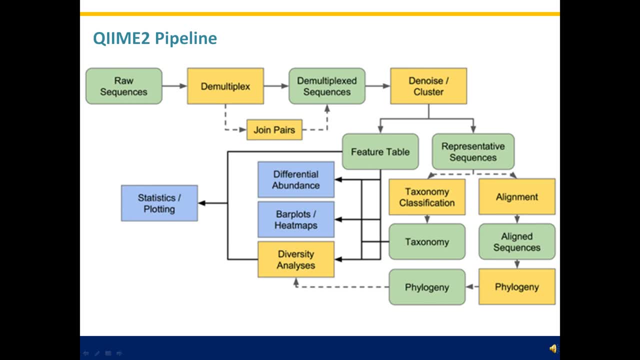 operation operation taxonomical unit will be at an genus level, so the accuracy will be more until genus level. so this has a oral pipeline for your microbiome analysis or metagenome analysis. so simply saying that once you get an raw sequences, just go for an demultiplexing if it is unpaired. and 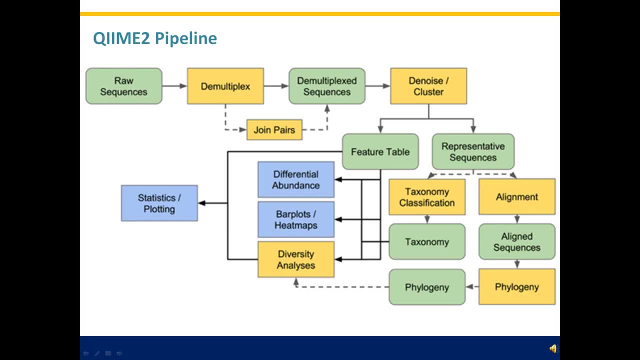 join the pairs and then make it as an demultiplexing, then going for denoising or clustering, then we are going to make and representative sequences, and these representative sequences will be used for building and phylogeny and as well as for taxonomic classification, by using and different kinds of and databases. 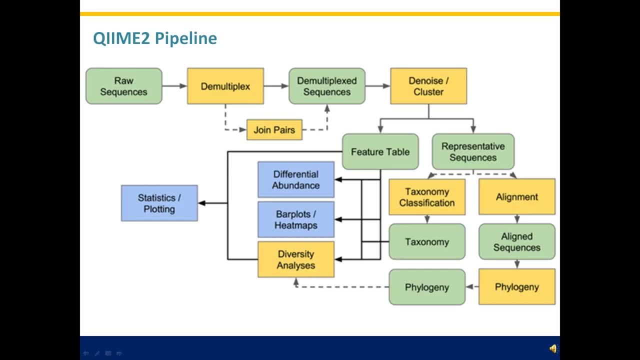 like our PD or silver or easy taxon. so once that axon, a classification has been done, we can make the different, we can see the differential abundance. or we can make an bar, plots or heat maps and we can study and diversity analysis like alpha, beta diversity analysis, and then we are going to plot that by you, we can. 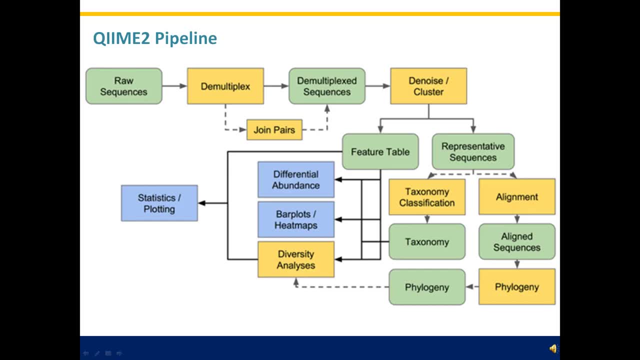 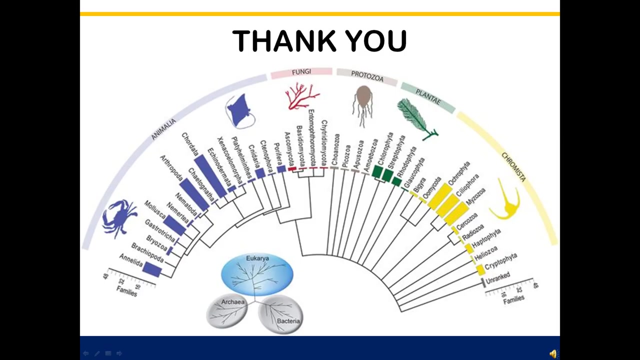 perform some statistics to know the significant difference, so by using an, our statistical tools. so this all overall summary of our time to pipeline so which we are going to study in further classes in more detail. so so this is what we are going to learn in this advanced environmental microbiology. so alright, students, this is all for today. 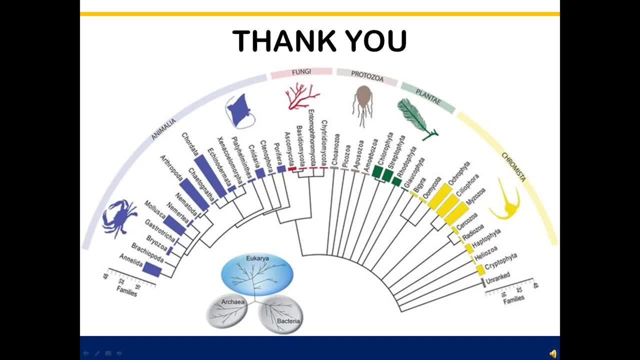 so in next, for the coming classes we are going, we will go more deep about each and every section of the course and we'll try to understand and so how the bioinformatics has been helpful for us to analyze the microbiome or metagenome data analysis from an environmental samples, and we'll try to understand what tools are. 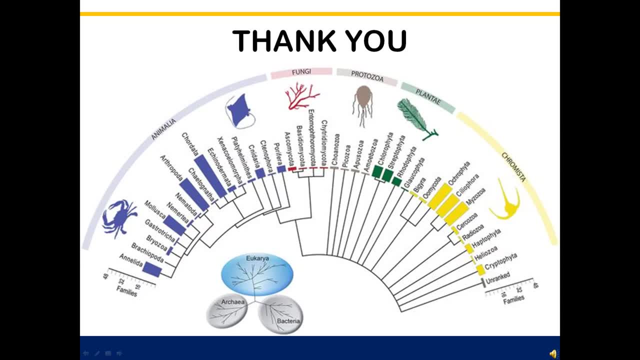 available for us to easily and how we can use them the best. so that's all for the class today, thank you. thank you one and all.